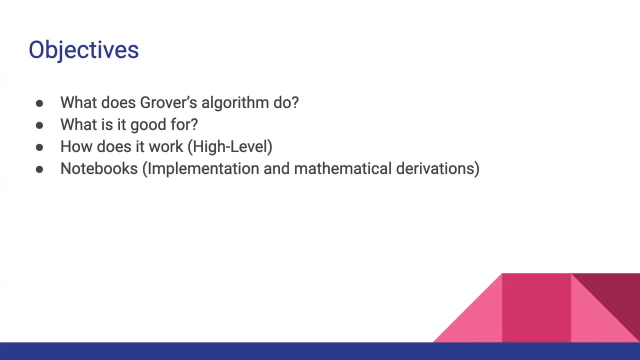 as well as all the other technicalities. So I have the objectives that I want to cover. Once again, I'm hoping to keep things hybridized So you have a code interactive component. It'll be something for you to mess around with and get a hands-on feel for, But in the very beginning, 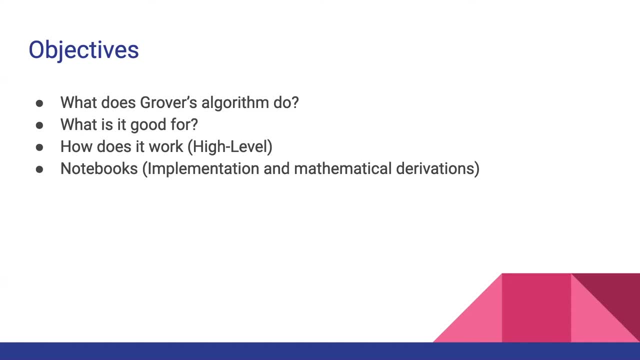 I'll give a high-level overview of how the algorithm works And I'll leave it to you guys to look at all the math and all the derivations, Because I used to doodle it on the on this little board here, And then I realized: one, my handwriting looks like shit. And two: 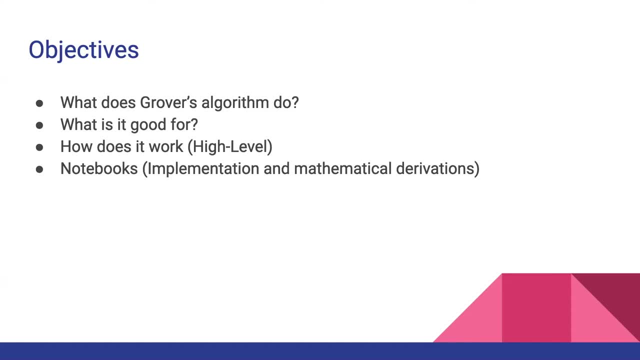 it's probably much more fruitful for you guys if I just give you the big idea And then I'll let you kind of munch on all the smaller tidbits there. So the goal is: what does Grover's Algorithm do? What's it good for? How does it work? So that's the high-level stuff And some of the Jupyter. 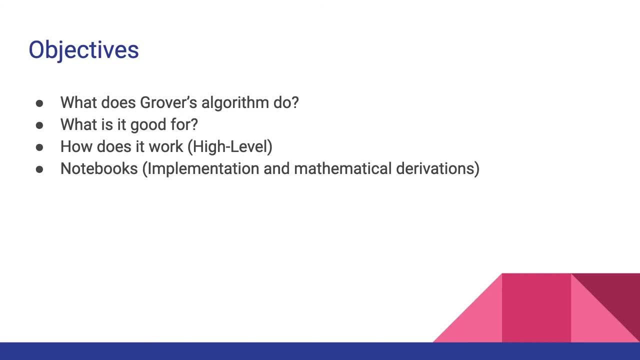 notebooks. So just like last time we had the notes of all the Deutsche Hose stuff, So this time around I have plenty of notebooks. by the way, I had a lot of stuff prepped. It's a shame there was a. I remember there's someone here saying they wanted more interactive stuff and they're not here. 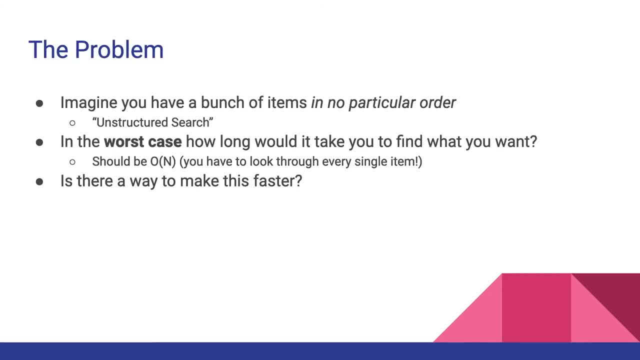 So, anyways, all of these algorithms are designed to solve some kind of problem. That's just the inherent nature of any algorithm, And the problem is so. let's imagine I give you a bunch of items and they're in no particular order. In fact, a lot of times, when you learn about Grover's 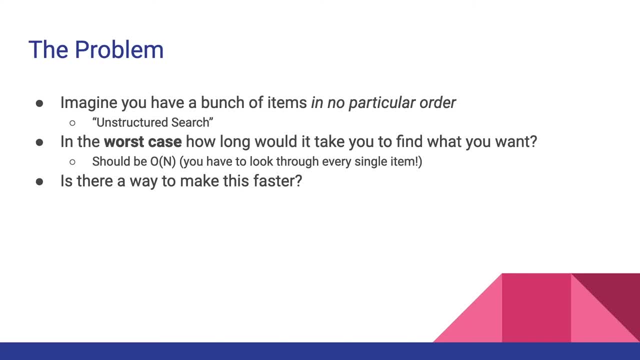 Algorithm. one of the terms they'll throw around very nonchalantly is unstructured search. So what exactly that means is all the items I've given you have no pattern to them. They're not or arranged in alphabetical order or numerical order or any sort of order, just randomly in a 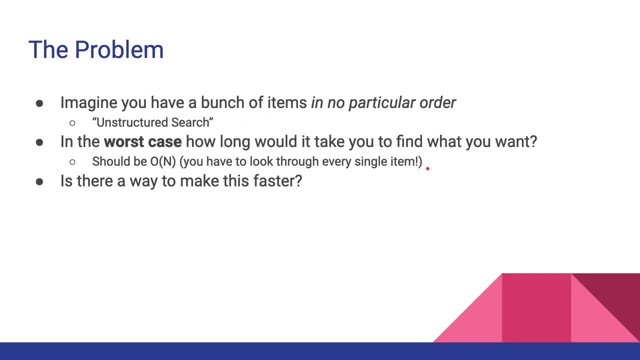 pile. So, in the worst case, how long would it take for you to find what you wanted? Well, if it's a bunch of random items, the worst case is you have to look at every single item to the nth item. That's what big O of n means. That's the worst case scenario. 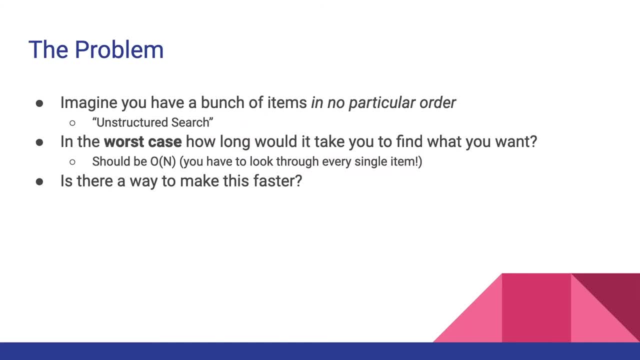 But now I ask: is there a way to make this faster And intuitively? this doesn't seem possible because at this point that's where the quantum weirdness kind of kicks in. And I can tell you that, yes, we can do better than the worst case scenario, which is like looking at 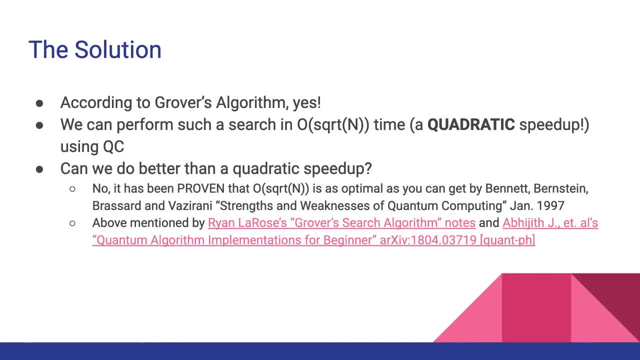 all n items. And yes, according to Grover's Algorithm, we do have a possible speedup. In fact, we can do it in O of square root of n, which is very weird because classically speaking, that's almost like if you only look at the square root of the number of. 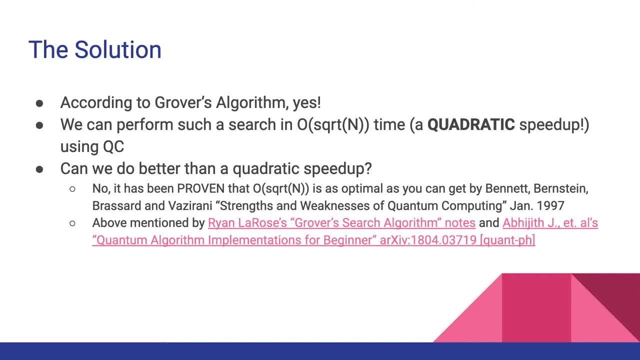 items in your stack and you can figure out like: OK, I just found the item I wanted which is, classically speaking, it's very odd. That's a quadratic speedup. And so you think: well, if it's a quadratic, how about, I ask, can we do better than a quadratic speedup? 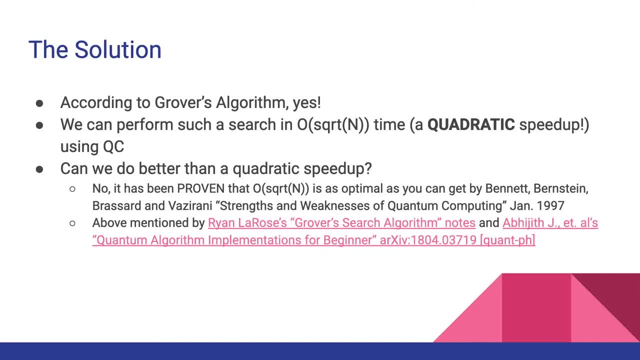 Because in the history of computer science what happens is someone finds an algorithm and then another computer scientist says like, hey, there's a trick we can use here. And it's the same thing in quantum computing too, even in the field of work that I do with graph. 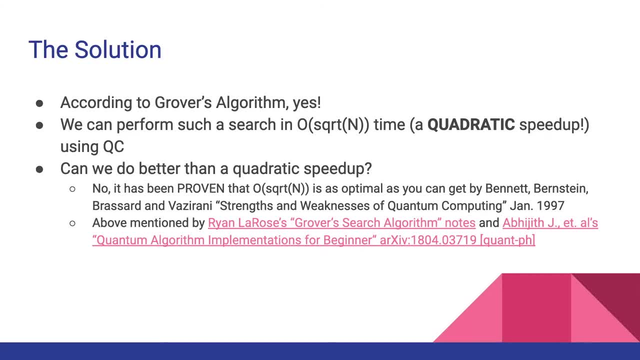 isomorphisms. It's interesting to see people iterate on that work and make faster algorithms that are more resource efficient. And it turns out that in January of 1997, there is proof that O of square root of n is as fast as you can get. 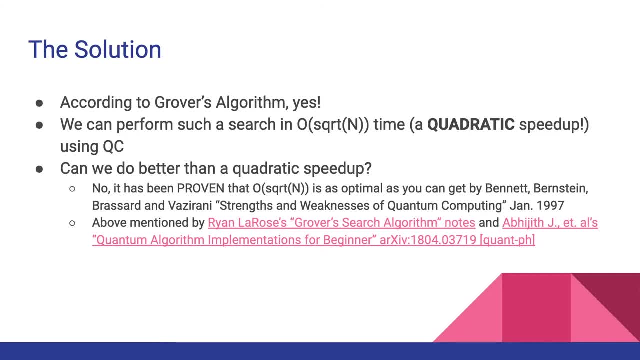 So you can go no further, no better than O of square root of n. If you're really curious about it and you go on Wikipedia, apparently there's a way to get O of the cube root of n, but that involves some kind of weird setup. It's like a minor footnote. I have to check the source on. 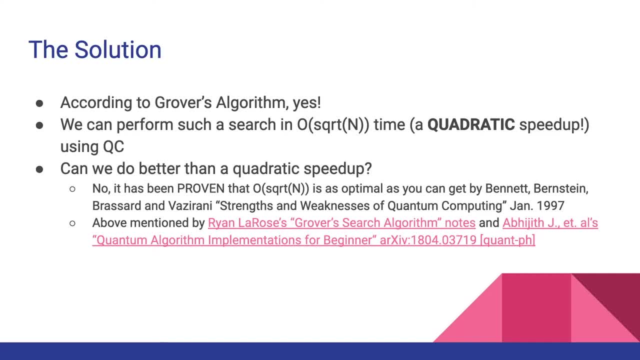 that Remember. when you're looking at Wikipedia, always make sure you double check those footnotes. And oh yeah, I have some sources for you guys. The slides will always be up on the website. I encourage you to look at these sources. I mean, by no means am I. 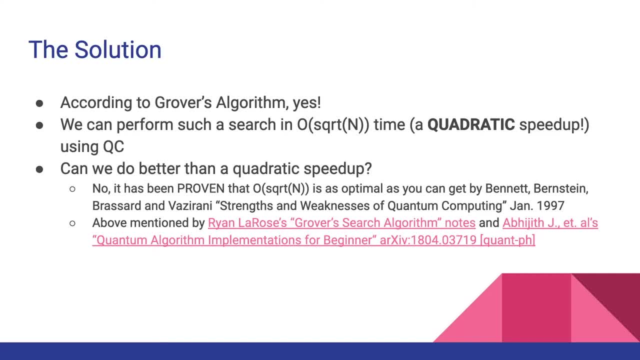 like the super genius here. I mean I'm consulting like 10 or 20 different sources to try and pick out the information I think will be most useful and most friendly for you to understand. So this is a formal definition of the problem. So in an unstructured search problem, 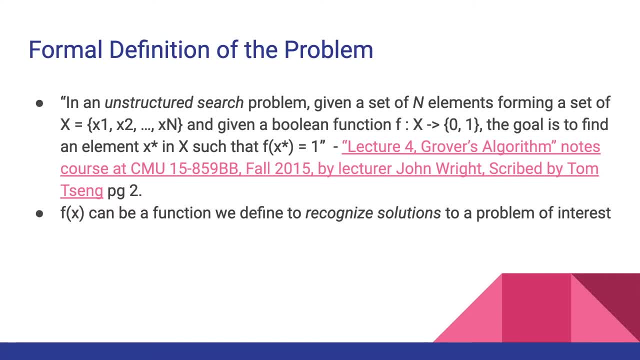 so, given a set of n elements forming a set of x, so from x1 to xn. so that's the bunch of random items I gave you, And there's a Boolean function. So all this function does is it takes any x and it gives you a 0. 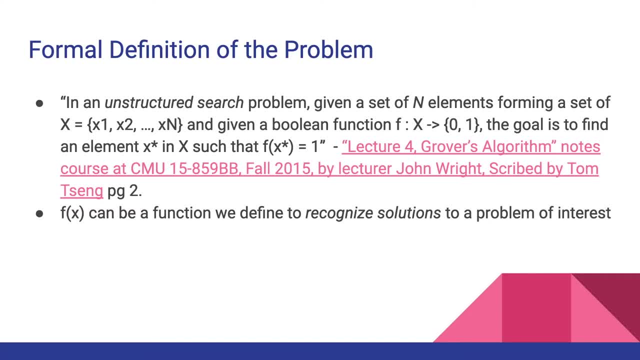 Or it gives you a 1.. The goal is to find an element, x star. So that's like the item we're looking for. That's the solution, And f of x will give us 1 if it's the solution and 0 otherwise. 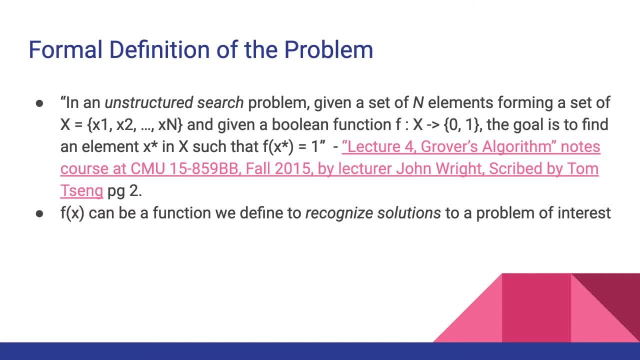 That's it. That's all f of x does, And I put this here on the bottom. f of x can be a function that we define to recognize solutions of a problem of interest. I remember in the very beginning there was someone on the Zoom call who asked because I brought up Grover's algorithm as a 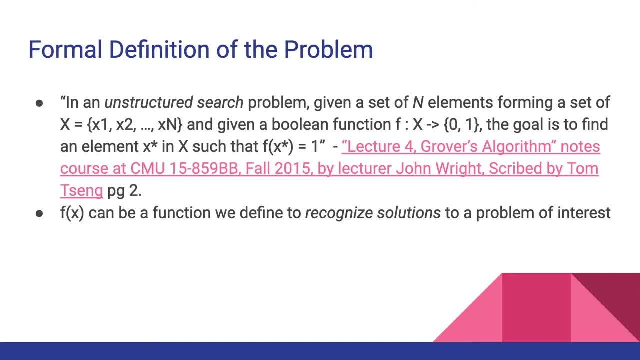 benefit of quantum computing. And he asked: well, wait a minute. It feels like in some of the examples for Grover's algorithm, that you already know the answer, So it doesn't defeat the point of having this algorithm. And it turns out that there is a distinction between having 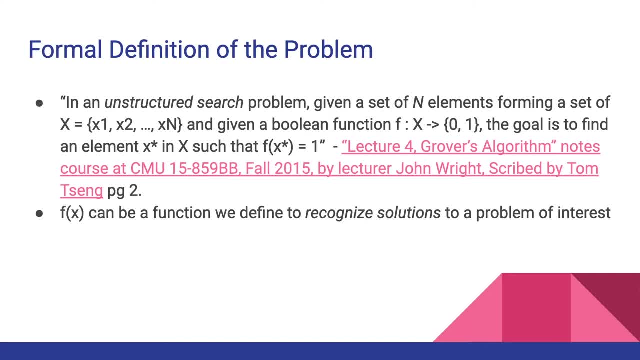 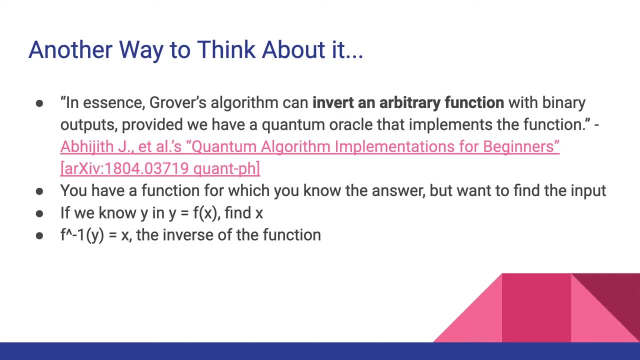 a function that calculates the answer and having a function that just recognizes the answer. So another way you can think about Grover's algorithm is we can take a function that takes some binary output and we can invert it. So if we have like, say I have y equals f of x and I know what y is, I can find what x is, So I can go backwards. 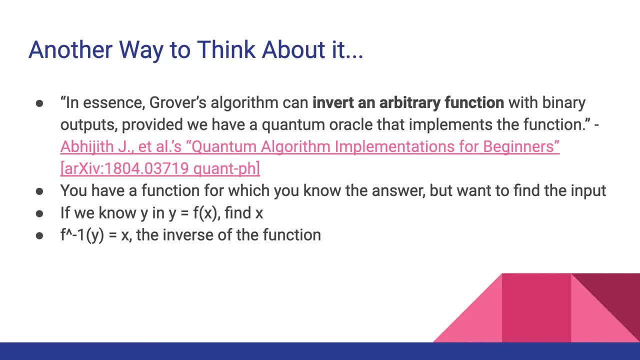 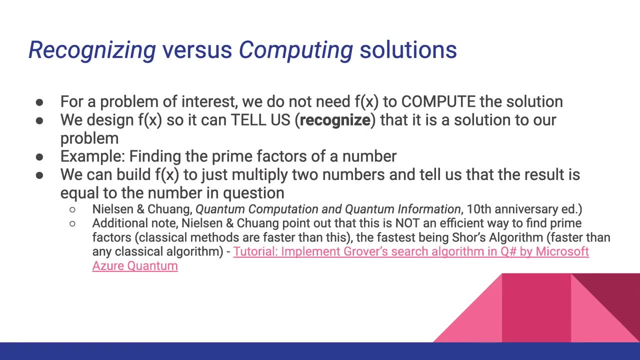 If I give you the answer and I need to find the x that gives me y, that can be done. Ah, OK, So here's what I was blabbering about earlier: recognizing versus computing solutions. So for a problem of interest, we don't need f of x to actually do any heavy lifting. 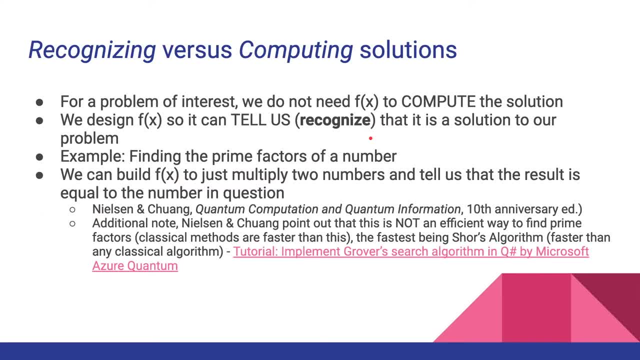 They're not too much heavy lifting, at least. Design f of x so that it can tell us that it's a solution to our problem. It doesn't really. it does some calculation, but it's supposed to be very efficient, Because all we're doing is. 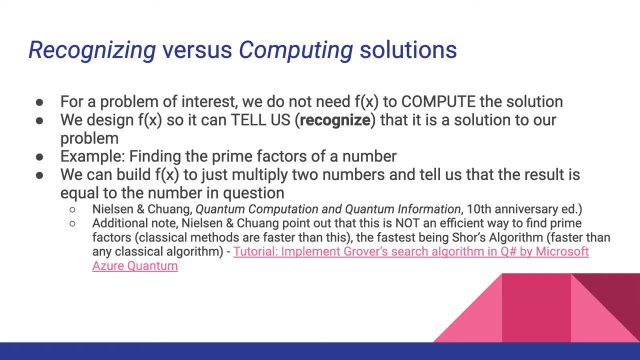 checking for the answer, And the example that I give you of the difference between computing and recognizing a solution is one that gets cited. Nielsen and Toine mention it. I think pretty much every source on the internet that talks about Grover's algorithm will use this. 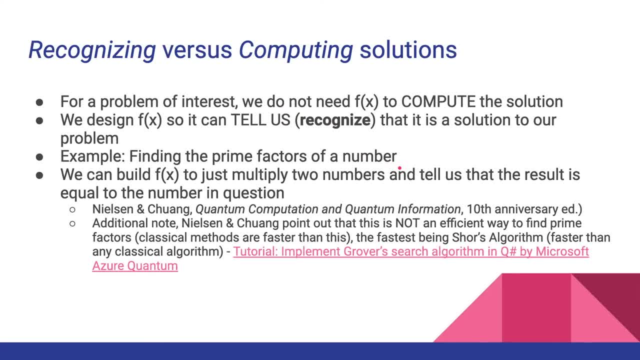 example, which is finding the prime factors of a number. So to just recognize that there are two valid prime factors, All that f of x has to do is multiply the two numbers together. That's a very trivial thing for a computer to do, even more trivial for a quantum computer. 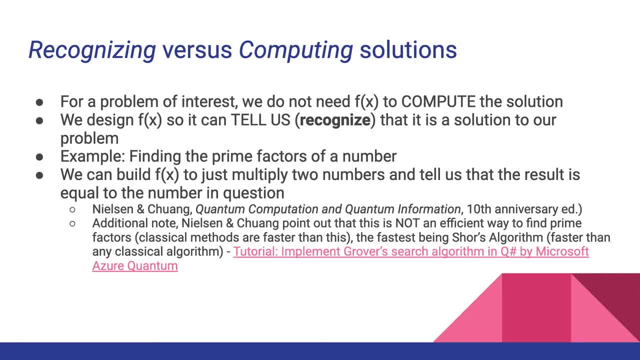 and easy for us to do, even on pen and paper. It's very easy to check if two numbers multiply to a bigger number. But it is significantly harder to figure out if I just give you the number to figure out the two largest prime factors for that number. But we don't need f of x to 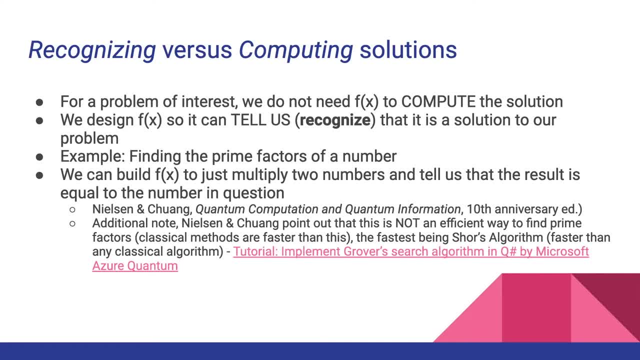 compute that for us We just need f of x to do the multiplication, Because another way you can think of Grover's is we're actually brute forcing That O of n, the worst case scenario where you have to check everything- it's pretty much the equivalent of brute forcing. I'm just plugging in. 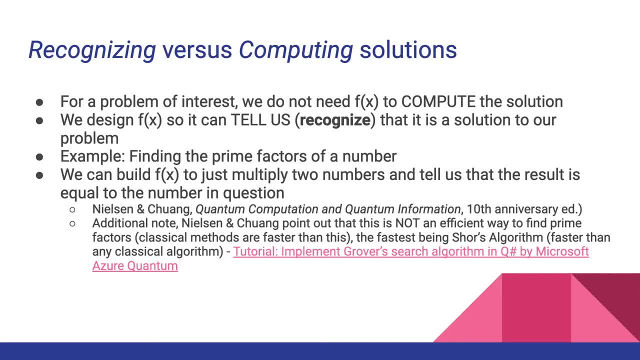 0 prime, not only 1.. And then you go all the way to n. It's kind of like that scene from one of the old Mr Bean movies where they can't tell the phone number of the kid So he has to punch in. 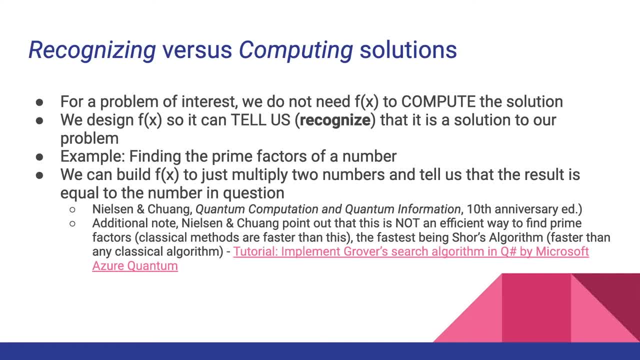 every single phone number And it turns out he actually misses the right phone number. So I waste all his time. I don't even remember the name of the movie. Anyways, I'm getting ahead of myself. The key point that I want you to remember is: f of x doesn't compute the function, It just. 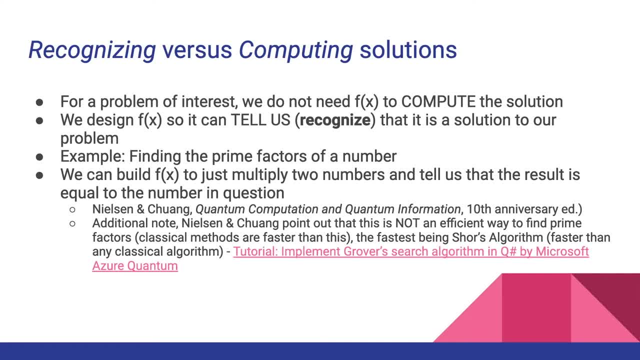 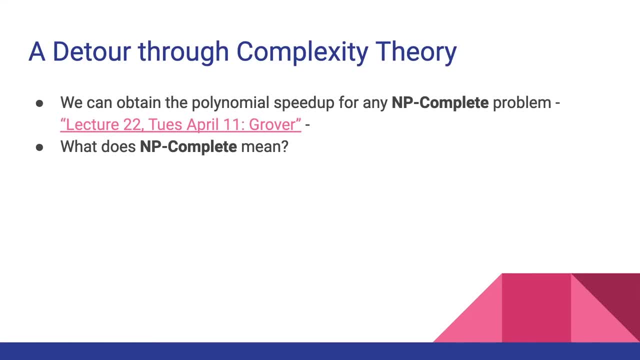 recognizes the solution, That solution will satisfy some criteria of interest to us. Ah, OK, So now that you kind of know what Grover's algorithm does, it lets us kind of invert functions, And, yeah, that's the right way to think about it. This is by Scott Aronson. Oh, 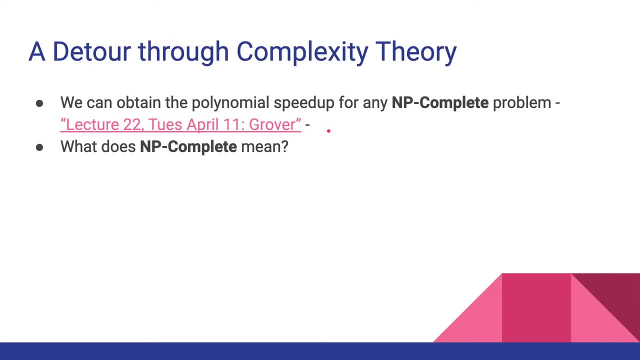 see, I'm missing the name here But the link's there. I'll give myself partial credit. But Scott Aronson says that we can obtain a polynomial speedup for any NP, complete problem. So the polynomial speedup. if you remember earlier I said worst case in our world is o. 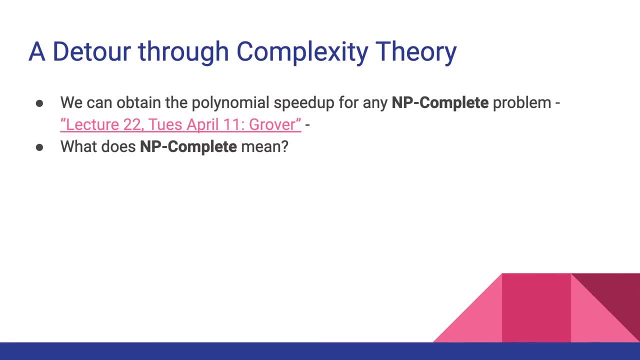 of n, But for the quantum computer it's square root of n. So we consider that a polynomial speedup And for any NP complete problem. if you come from a computer science background, NP, complete, NP, p, all that stuff is very familiar. But I know we have a. 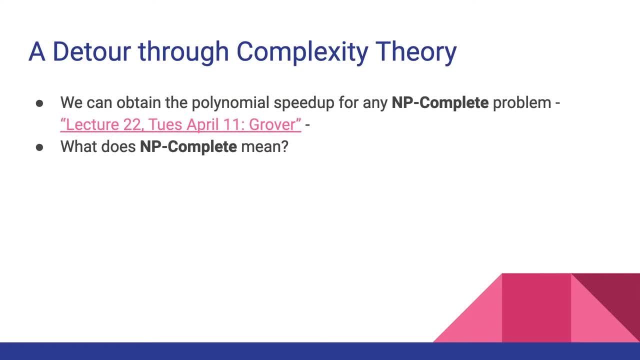 very interdisciplinary audience And I think it's worth taking some time to explain. what does NP complete actually mean? So that's why I call this a detour through a complexity theory. So if there's one thing that people in CS love, it's categorizing problems, And people in CS 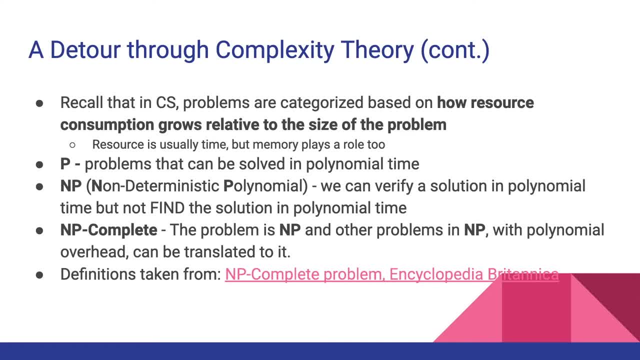 categorize problems based on resource consumption growth relative to the size of the problem. So what I mean by that is if I make the problem some unit larger than it used to be and I look at how the time grows. Time is a resource. Memory is a resource. The most popular is time. But 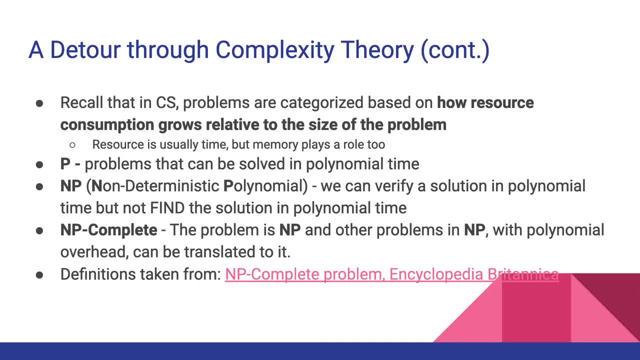 memory comes up as well. In quantum computing we care about the number of gates, which is almost like the equivalent of number of operations that the quantum computer needs. So for problems in P we say that they can be solved in polynomial time And you can find a solution. You can verify the 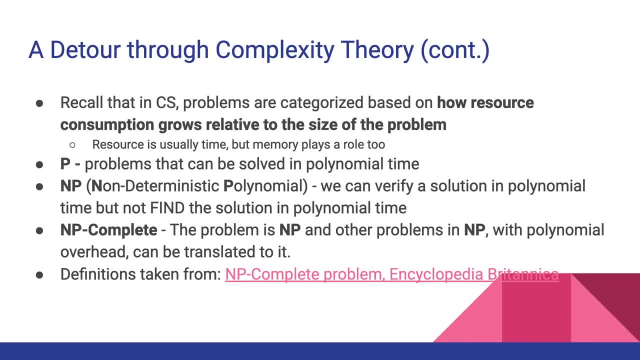 solution in polynomial time as well. It's very easy stuff: NP. that's what NP means. by the way, NP does Not mean not P. I thought that was a situation for the longest time. It turns out it means non-deterministic polynomial. Don't worry about where the non-deterministic comes from, That's. 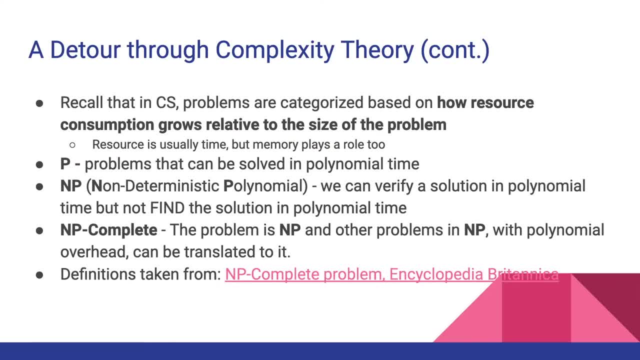 another area of CS theory that I'm intentionally protecting you guys from. You can go down the rabbit hole, But the idea is that you can still check if the solution is correct in polynomial time. But I can no longer guarantee for you that we can find the solution in polynomial time. 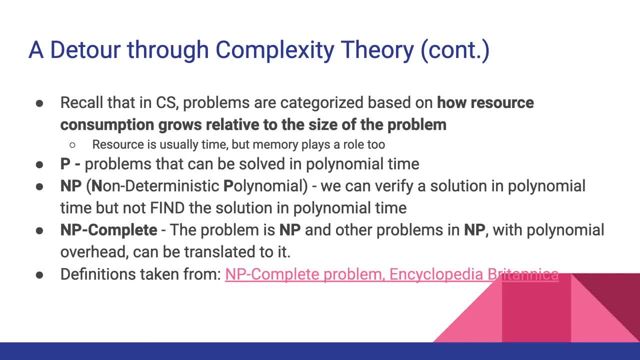 So we consider that NP, NP. inside NP we have problems that are known as NP- complete problems. So what that means is the problem itself is NP, But if I give you a little extra time, you can translate any other problem in NP to that particular problem. So you have: the problem is in NP and there are other problems in. 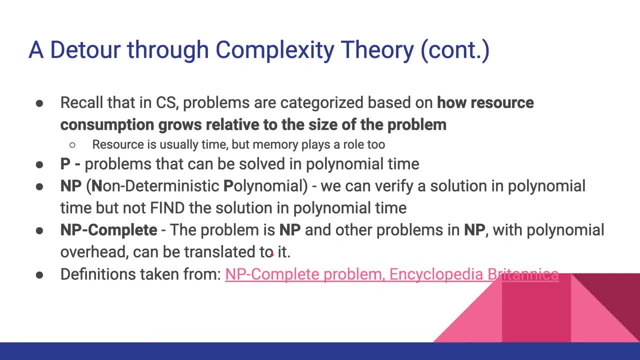 NP, Then with some polynomial overhead I can translate one problem to the other problem And you might think, well, what's the benefit of doing that? Well, if you have an algorithm that may solve that NP complete problem pretty efficiently, then it might be worth translating. 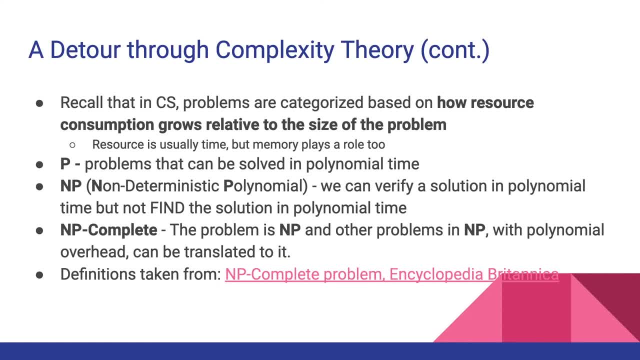 your other problem, that's NP, and getting it into the NP complete problem. That's the hope at least, Although the interesting thing is if there were a way to calculate one NP complete problem efficiently. it turns out that all the other problems in NP kind of collapsed in terms of 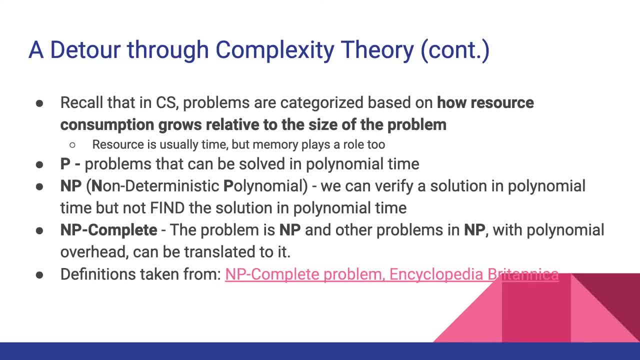 complexity, And it's the very famous P equals NP question. Because of all the other problems in NP, a lot of computer scientists for decades have asked whether or not it's possible that the problems in P and the problems in NP are actually the same category. We haven't figured out. maybe 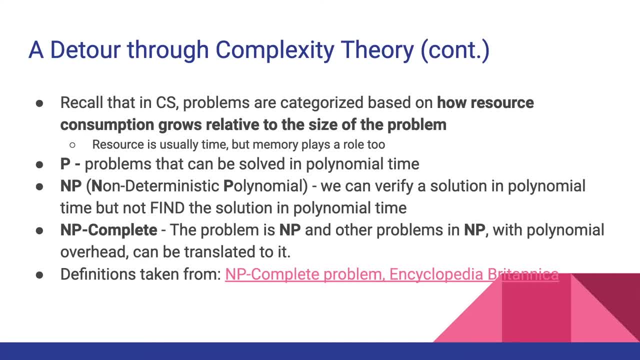 because all you need is one problem. All you need to do is figure out how to solve one problem in NP efficiently, And then the whole thing turns all into P. But for the past several decades we haven't been able to figure that out. So that's an open question. It's not even on my 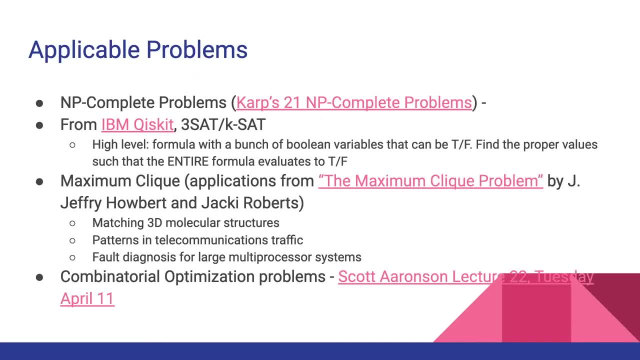 slide. I'm getting ahead of myself, But it's something I think is very cool. So here's some applicable problems. I mentioned NP complete problems. If you don't know who Karp is another famous computer scientist and not a fish, But Karp has a list: 21 NP complete. 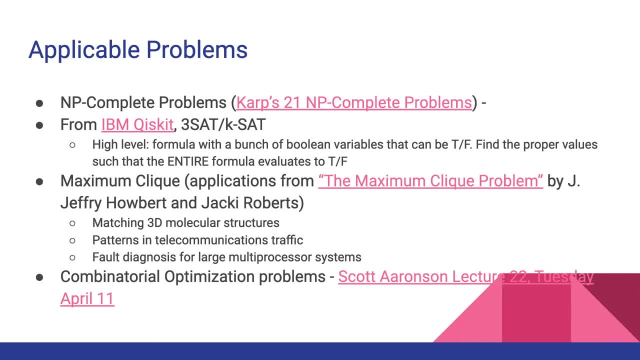 problems. So I think he published this in the 70s And this is the first case of all these NP complete problems. And NP complete doesn't really make much, doesn't have much of an impact to us as normal people. Well, I'm not saying people who work in quantum computing are. 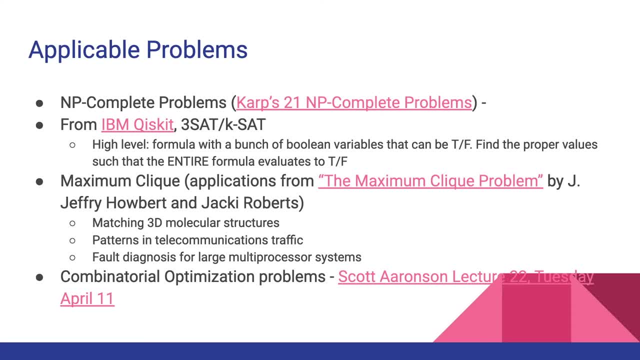 computer scientists or weird or anything. But a lot of problems you see in industry, in science and technology and once again they have their roots in being NP problems or NP complete. So if we have a way to efficiently solve these problems then it's kind of a benefit that. 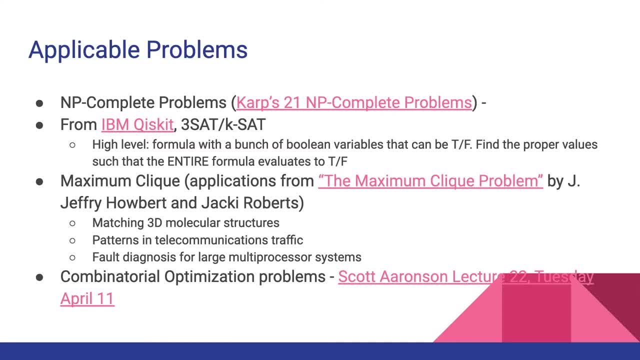 can spread out. So from Qiskit and the example that I want you guys to investigate is known as 3SAT or KSAT, And the idea is we have some kind of formula that has a bunch of Boolean variables. So Boolean just means it can either be true or false, And the idea is I can string a bunch of 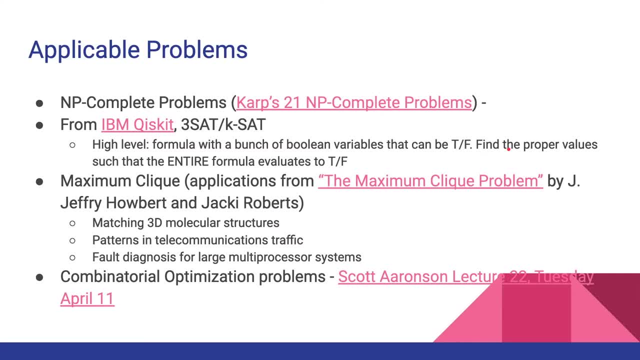 these variables together So I can say like X and not Z or Y, just string a bunch of them together And that can represent in industry a lot of optimization problems. I think scheduling is one of them. I'll have to pull up a source to be sure, But SAT and KSAT come up a bunch. 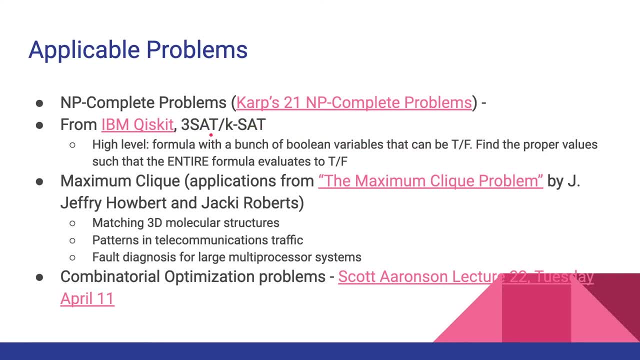 The reason for the difference in number here is these Boolean satisfaction problems have a certain format And the number is a certain format, And the number is a certain format, And the number is a certain format, And the number just represents, like you can think of it on a high level just. 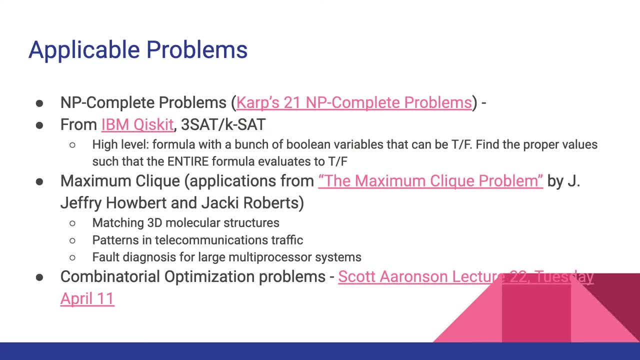 how many variables you can lump together in one term almost. There's also the maximum clique problem. Maximum clique- I don't know how familiar you guys are with graph theory. I can make this quick. So if you imagine, let's imagine we're all like in a group of friends. I know it's weird. 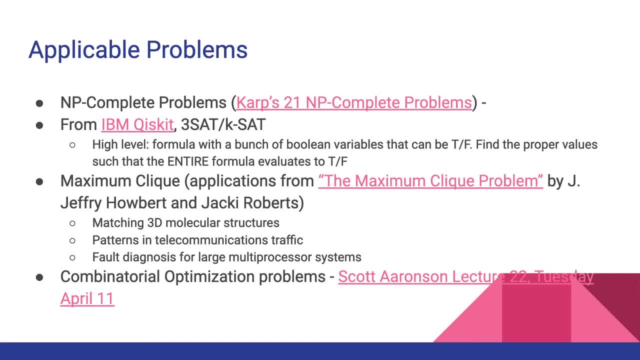 but just bear with me here. So we're all like a nice group of friends And it turns out that maybe we're all in a group of friends And we're all in a group of friends And we're all in a group of people And it turns out that maybe out of all of us, four of us consistently talk with each. 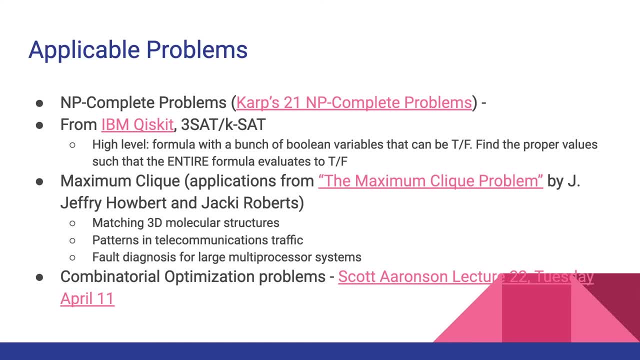 of the other three people in that set of four. So that means we consider that a clique. It's when, like all the elements are connected to each other. Every other node is connected to every other one. A maximal clique, or a maximum clique is the largest clique you can get, Because you can have. 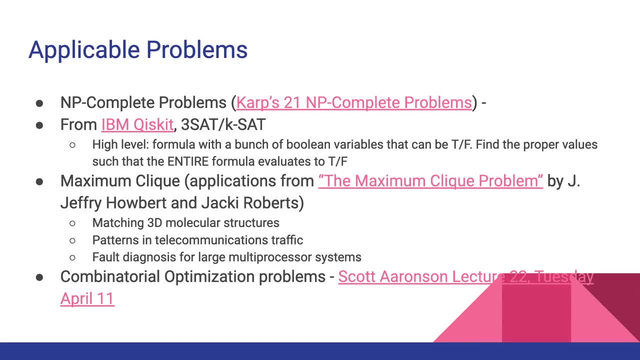 a clique of three nodes. It's a triangle essentially, But it's a small one. It's not the biggest one. So out of out of our group of people, if we had like a clique with you know people. so that means that every, every person has a connection to all the other four people. we 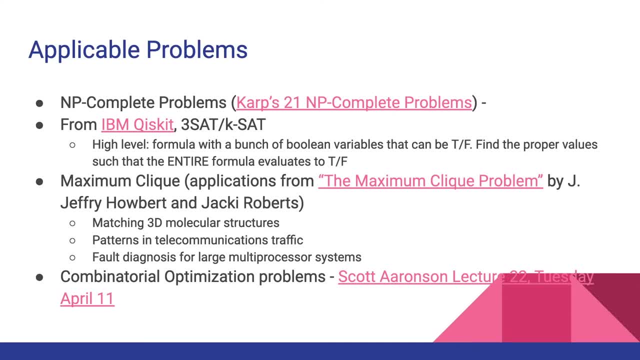 consider that a maximum clique. that is an empty, complete problem, and it turns out that it has the following applications, such as uh matching, 3d molecular structures- that just comes up in pharmacology- uh patterns and telecommunications traffic, so like on social networks- um, that's like. 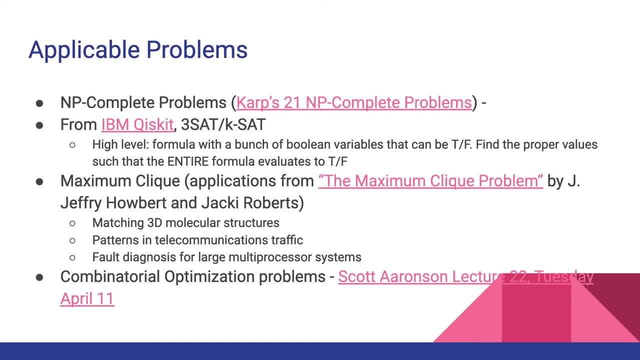 the kind of the friend example i gave you. i know facebook is probably doing millions of you know cliques and recommending you um friends i i would assume that's part of their algorithm and a fault diagnosis for large multi-processor systems. i'm not even quite sure how that works, but 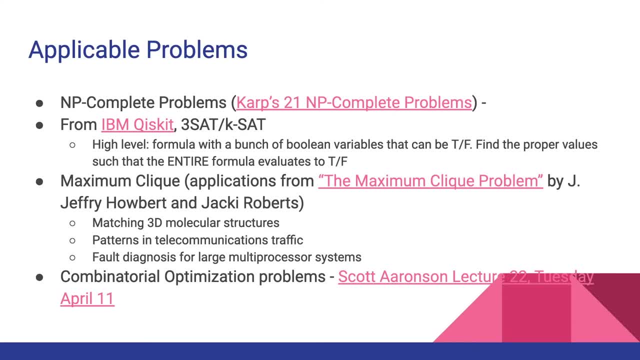 it was in the report that's been cited here- and the combinatorial optimization problems, um, this is a an area that i'm very familiar with, just because my work is in. uh is sort of is sort of related to that field, but the basic idea with co problems is um, 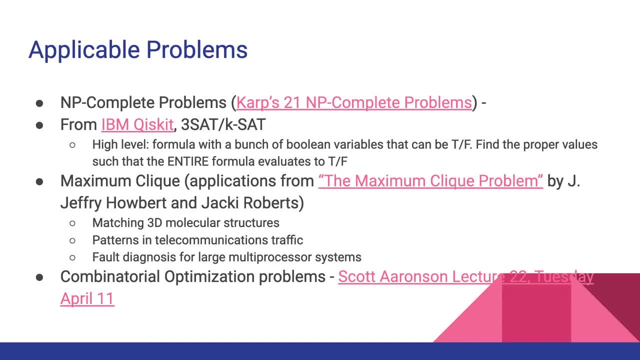 if i give you a set of objects and there's some optimal way to pick from that set of objects or to arrange that set of objects, we consider that a combinatorial optimization problem. so a grover's algorithm can provide a speed up for all of these problems and it's a 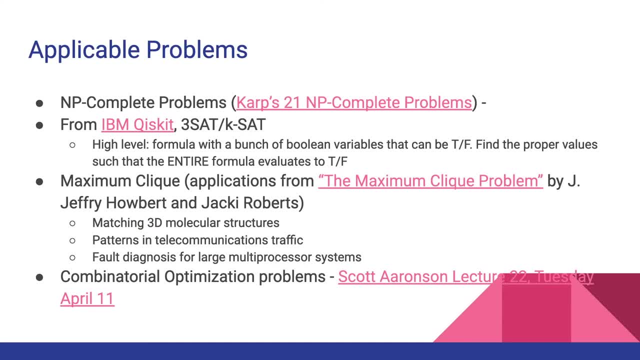 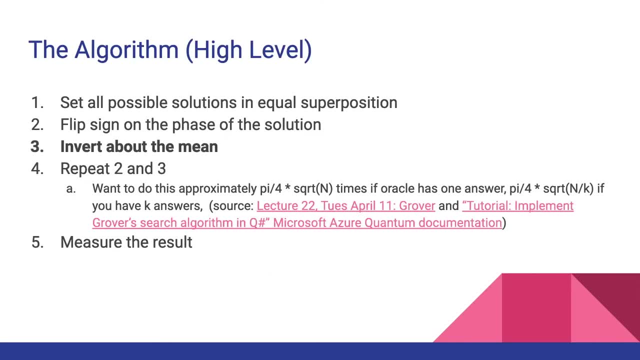 speed up. it's not meant to. it's not going to make p equals np. it's not going to happen with grover, but it is. it's nice to have. so i'm going to give you an overview of how this algorithm works. it's, it's a particularly elegant algorithm. in fact, i um, uh, it's, yeah, it's, it's really nice. 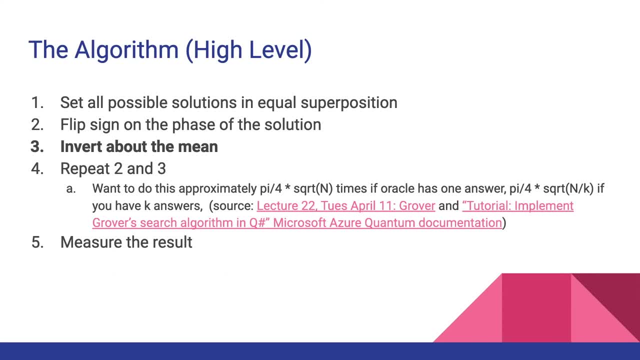 too. what am i mumbling about it? it is, it's a nice algorithm. so in our first step, we're going to set um all the possible solutions in in a equal superposition. so if you remember, george hosa, what we did was we just put a bunch of hadamards, and the hadamards were 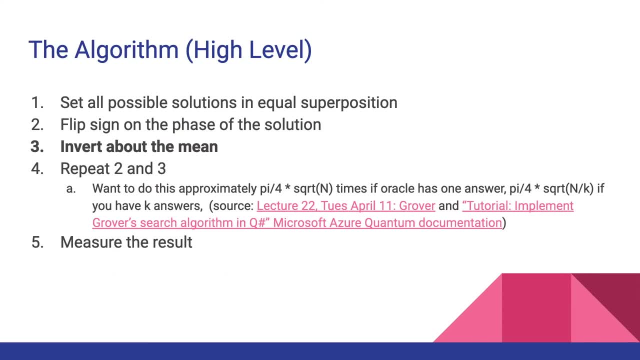 starting from from the zero state, so all the qubits are in zero. slap a hadamard on it, it becomes like a one over the root, two zero plus one over root two one. so we get them. so there's an equal chance. all these answers have an equal chance of showing up. now we're going to have an. 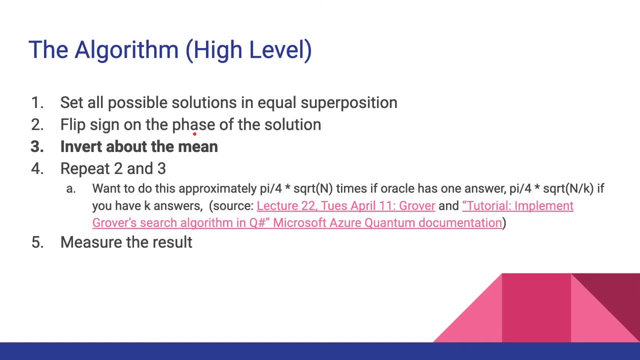 oracle and the oracle. once again, the oracle is the function i was talking about. the oracle is going to flip, going to flip the phase of the solution. don't worry if all of all this stuff i'm telling you right now doesn't really make sense verbally. i have pictures, so, um, you'll have something that's. 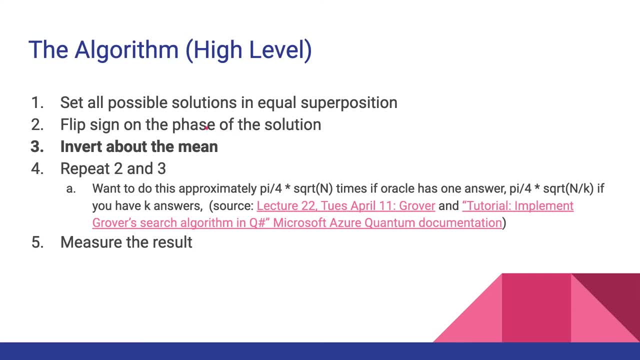 nice for your um, i guess your visual cortex- to munch on. now. this is the heart of grover's algorithm inversion about the mean. that's how we actually get the um. we get closer and closer to the right answer. and the way you define closer is that the probability of measuring the answer. 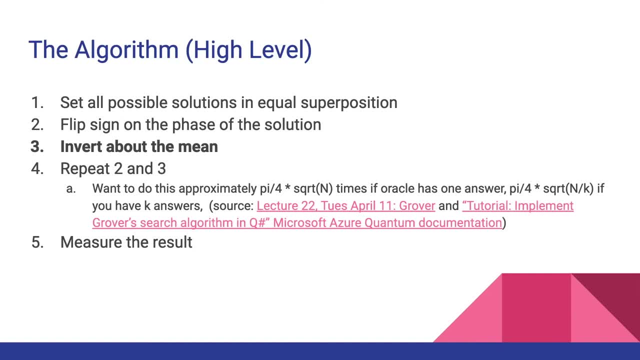 increases, whereas the probability of measuring the wrong answer is decreases. so we squash the other ones and we let the, the one with the higher chance, come up and we're going to repeat. we repeat, two and three, rinse and repeat, so you just, you just keep applying it um and there, but you don't want to apply it forever. it's not one of those. 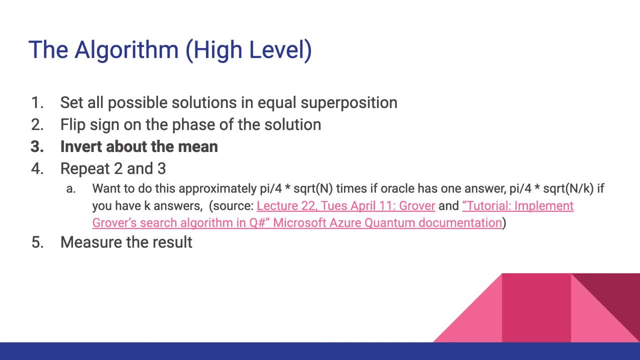 algorithms where you let it run longer and longer and you get closer and closer to the answer. in fact, it turns out, uh, i'll get to the caveat section. there's a bit of a. it's a bit of a problem when it comes to running grover indefinitely. i won't spoil it now, um so so. 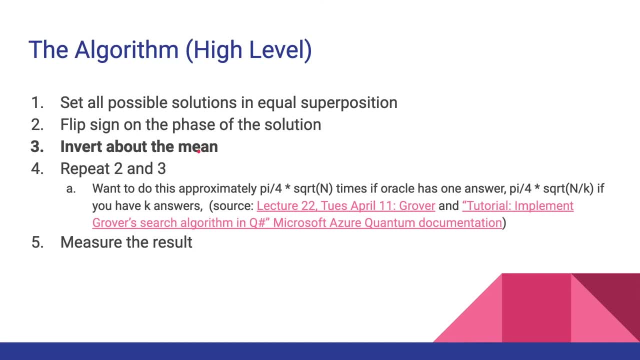 how many times should you run? you know two and three. if i say rinse and repeat, two and three, and rinse and repeat, and i say like, well, it's bad to let it run forever, it turns out you run it approximately pi over four times- uh, the square root of n times. and if you're wondering where, 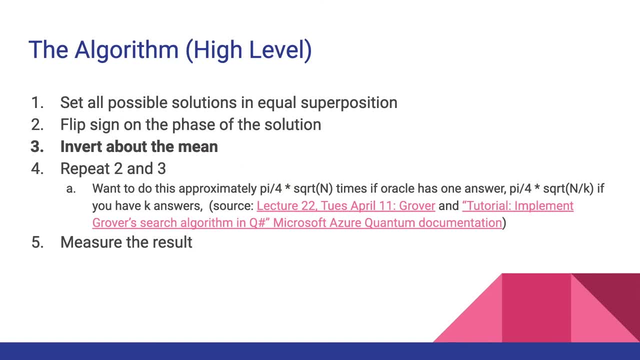 that comes from. it's a very weird number: pi over four to this times the square root of n, it turns out there is. there's something that i omitted from this presentation and from this workshop. there's a geometrical interpretation of grover's algorithm, um. where you can, you can represent um. 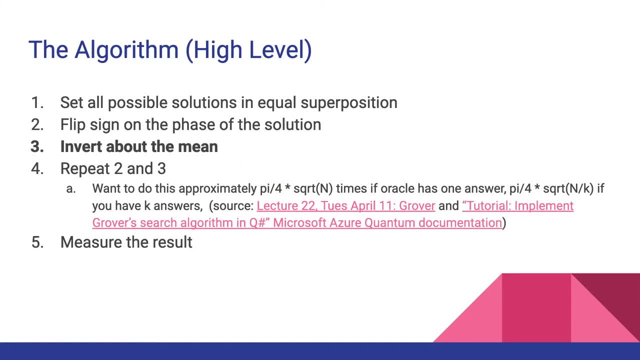 the system as like two vectors and you do a number of specialized rotations and you rotate to the correct vector. answer that's. that's a geometrical view. i opted not to show you guys that because it's just um. i wasn't too happy with all the answers. i all the presentations i found. 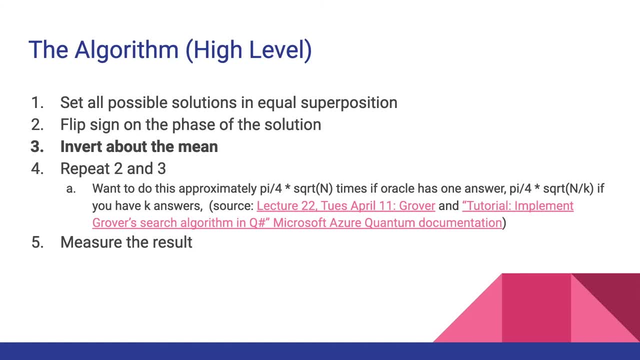 because i'm not going to teach you guys extra trigonometry and stuff like that. and, quite frankly, i think, um, i think the explanation i'll give you will be sufficient for your purposes, but uh, yeah, and then at the very end you perform a measurement, so we're going to destroy the 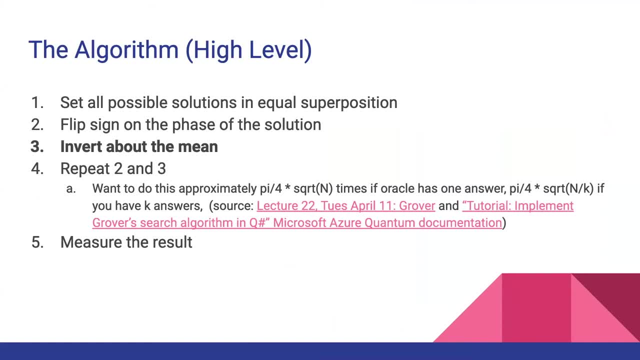 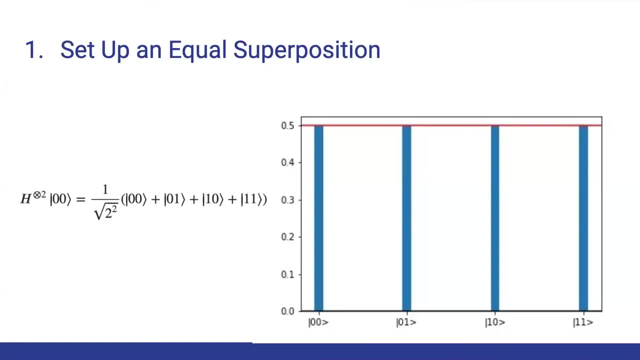 superposition state and ideally, at the, at the measurement, we will get the right answer with a very high probability. so let's go ahead and look at those pictures i was talking about. they should be um helpful. so 650, okay cool, um, near the end i'll give you time to just look at the notebooks. 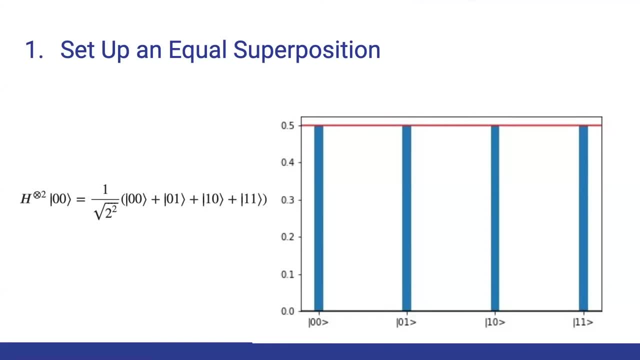 and um and if you see, like the rendering error i saw earlier, let me know i can push out a fix like right now. so in this particular case i'm only doing two qubits. so that means we have a total of four possible answers to look at. so when i apply the hadamard and we go from from the zeros, 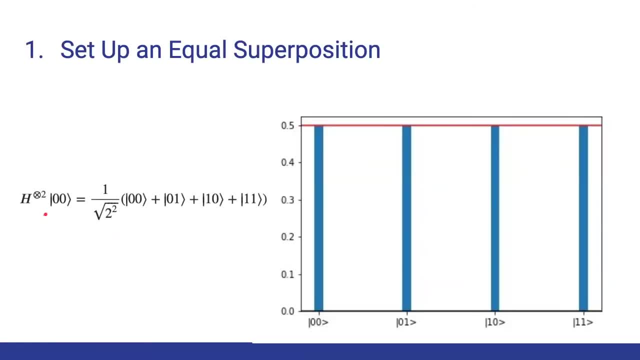 whoops, hold on. uh, i'm trying to laser pointer. so we go from the the all zero state and now every answer has an equal chance of showing up. in fact, these are what the bars show on the the 0.5 is i. all i did was i took the um, the uh, probability amplitudes here and i i graphed it out. 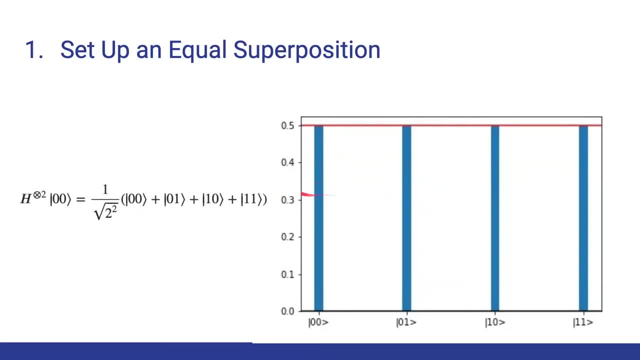 so um, so yeah, so they're all at equal um, equal chances. the red bar here is what i want you to pay a little attention to. that's the average. so i took all the um, like this, one over, uh, square root of the right side of the graph, and i took the one over two plus one over two plus one over two plus. 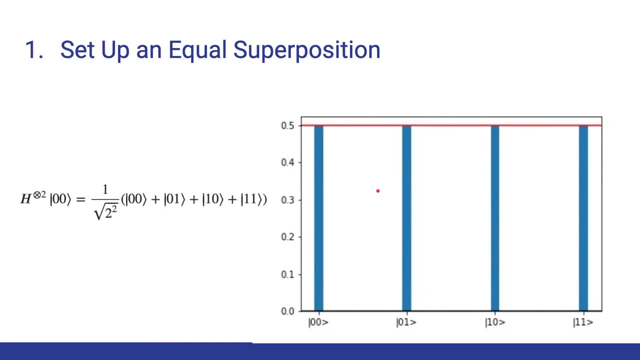 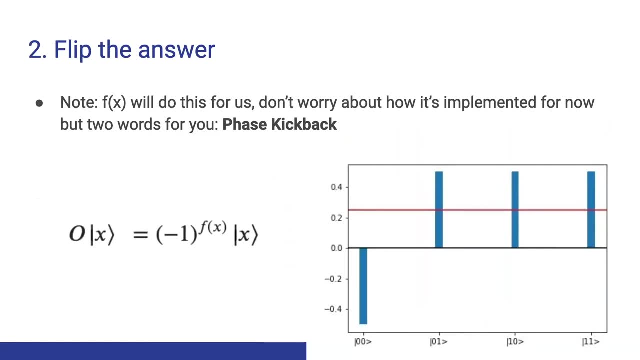 one over two and i took the average of that. so right now you know nothing, nothing fishy so far. it's it's a home territory. now i'm going to apply the oracle and the oracle recognizes which one of these inputs is. the is the correct answer. 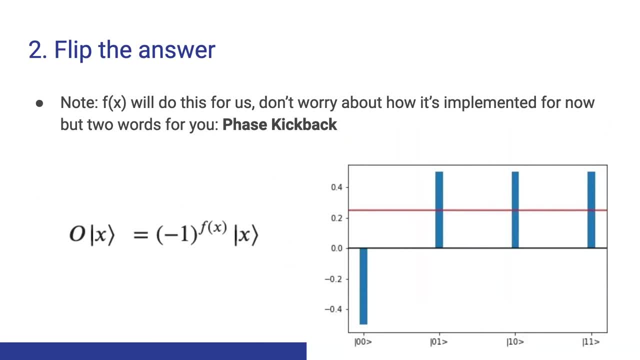 and what it's going to do is it's going to flip. it's going to flip the face. so in the beginning we were all all positive valued amplitudes. now i picked zero as the answer here. um, now you notice that the oracle is, you know, facing the other way. it's been flipped upside down, whereas all the 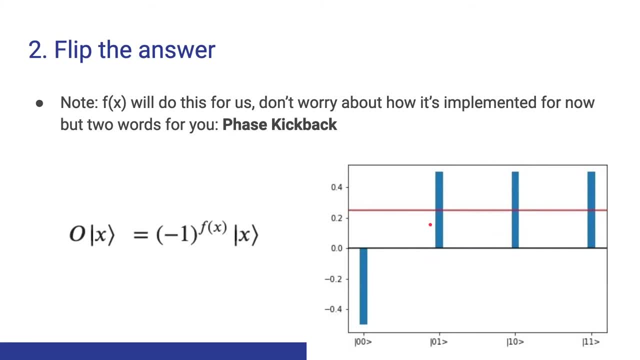 other ones are um still in the same position they were, but you'll also notice that the, the mean, the mean of the amplitude, has been reduced. so earlier it was at 0.5 and now we've brought it down to, you know, in between 0.2 and 0.4. if you don't know how, how the um oracle does this um, and this is why i. 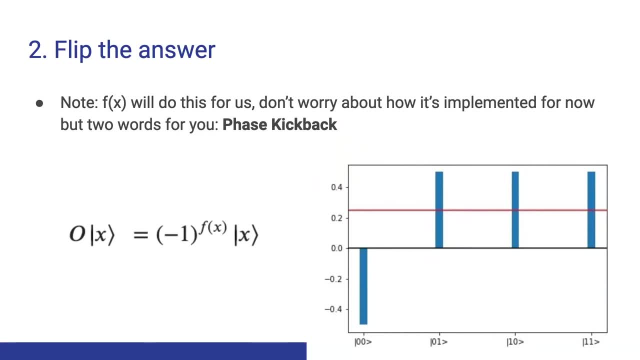 was, like you know. you're probably wondering like: why did john like say like phase kickback 10 million? why? because um in grover's algorithm we use phase kickback to literally um apply a negative phase to the target answer, so this notation should look somewhat familiar. this is um. i use this in the 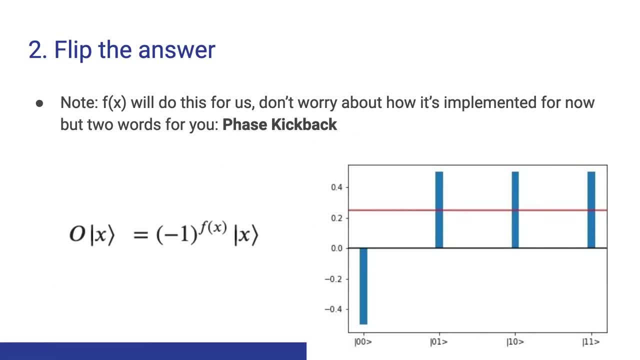 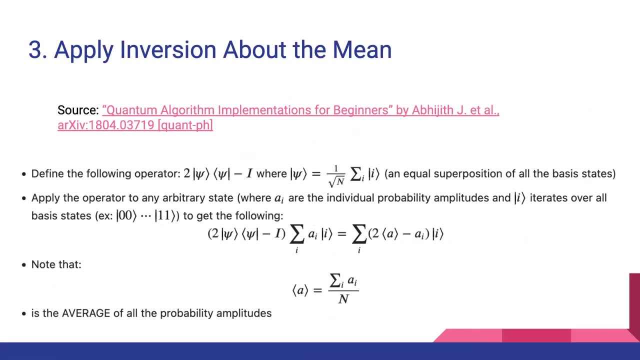 deutsche example. so we flip the answer and you notice the mean. the mean has changed now. so now we get to do the fun stuff which is applied version about the mean. and don't worry if the the math here like. i don't expect you to digest or even make sense of all the math, but i will. 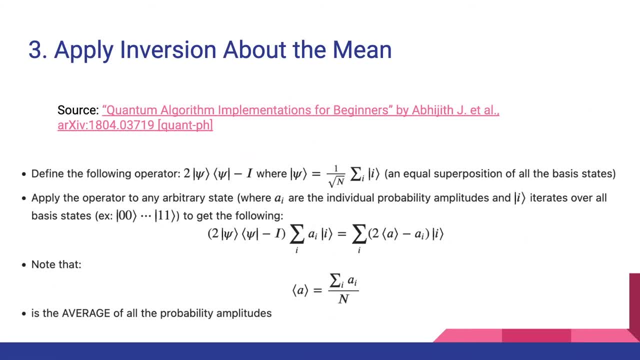 point out what i want you to understand, so to go into the the here, and that we're going to operator, to an arbitrary state. So in this case, the arbitrary state in question is in the summation here, because you can represent any quantum state as just. 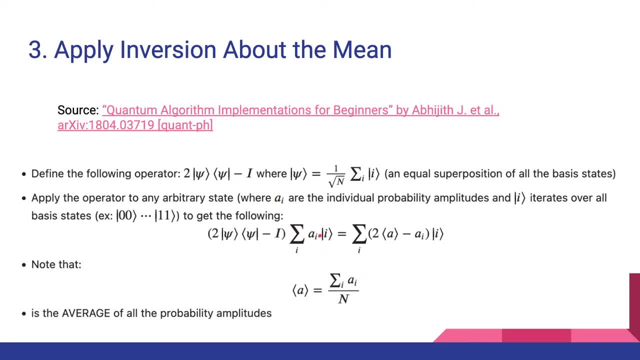 the sum of your basis states, And I want you to pay attention to what happens to the a sub i here. a sub i is the probability amplitude in front of that basis tet. The a sub i goes from just being whatever the hell it was. 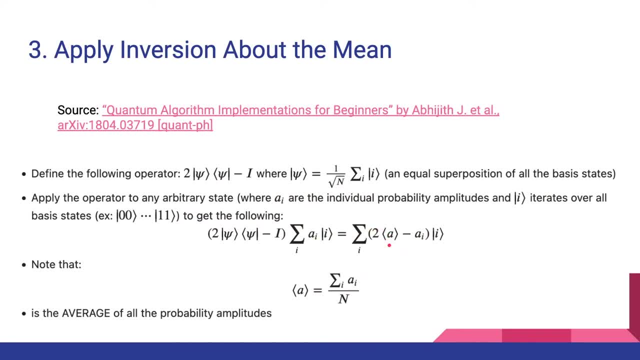 And now this thing gets applied, It's 2 times the mean. So you remember earlier that red line is the mean. So multiply that times 2. And then we subtract the older amplitude from it And this will literally flip. It's going to flip our values over the mean. 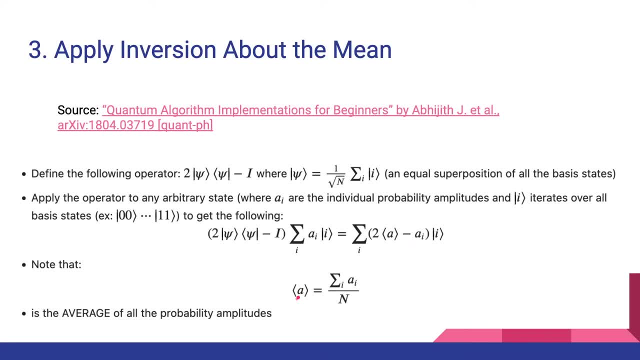 So inversion about the mean And yes, so note that the a with the two triangles on the a. that's just how we denote the average of all the probability amplitudes. And if that still sounds very abstract, don't worry, I've got plenty more pictures. 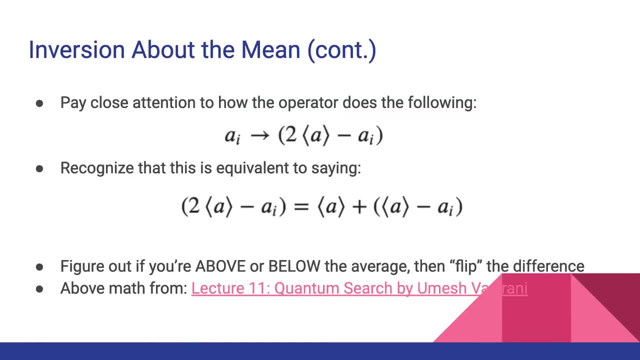 When I first learned it, it sounded pretty abstract. So yes, so this is what I was talking about. So this a sub i? a sub i is the probability associated with a certain answer. And then, when I apply the Grover operator, 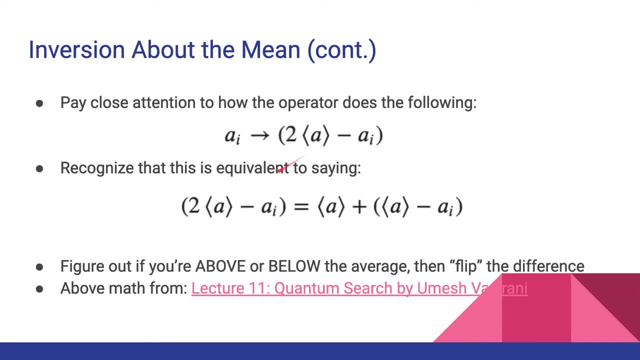 it turns into this: or 2 times the mean minus the amplitude, And I want you to recognize that this is the equivalent of saying this. There's no disagreement there. All I did was I split the mean like this, But you'll notice that now you can see better. 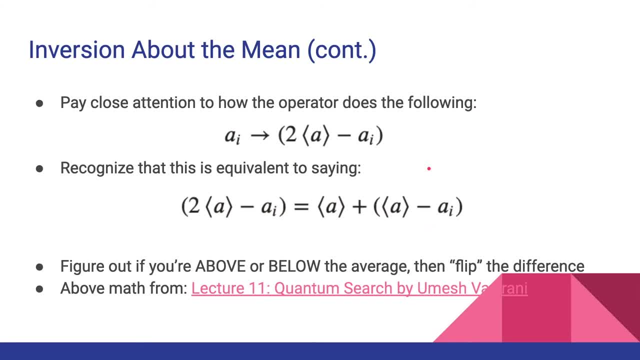 what's going on here? You take the difference from the mean and then you add it back to the mean and you get your new amplitudes. Just take the difference, Add it back to the mean. That's all we're doing. 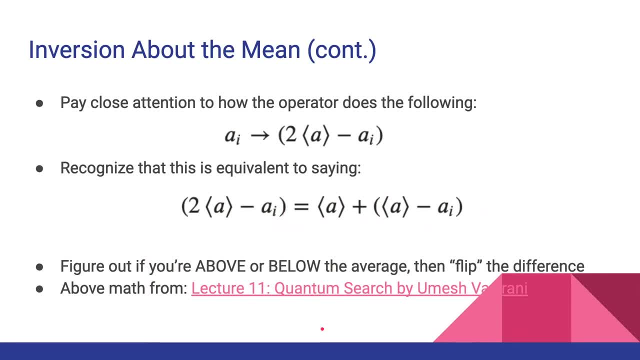 And so I took this little trick. It comes from Umesh Basarani. actually. Basarani is one of the huge names in quantum computing, And he has some YouTube lectures online. I don't think he uploaded them, though. It's kind of fishy. 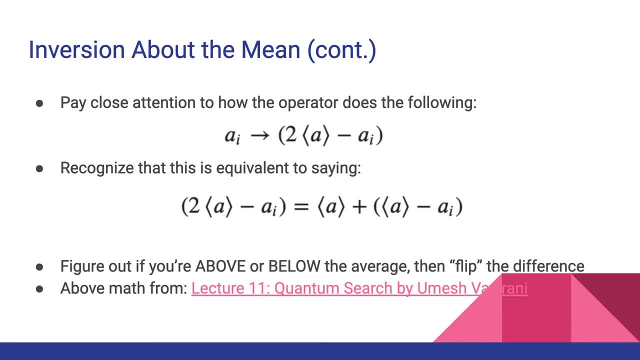 But they're up there. So I encourage you to check it out if you can, And so notice here. I said: figure out if you're above or below the average. So what I've done is I've broken down the different cases And we're going to see how the operator behaves. 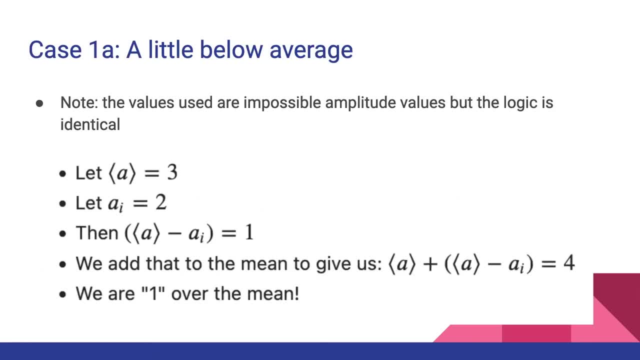 on those different cases. So case 1a: we have a probability that's a little below the average. It's not less than 0.. It's not negative, It's still positive, but it's just a little bit below 0.. 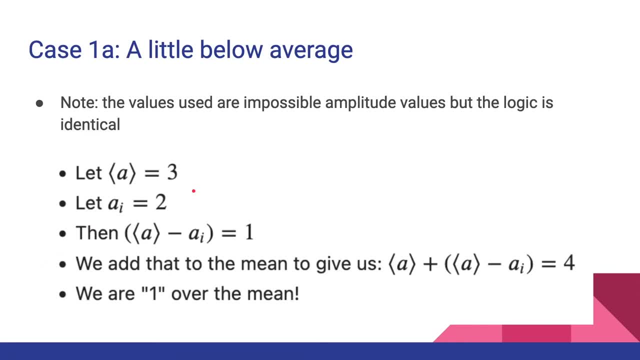 So these numbers, by the way, are impossible. If you have a quantum state that has numbers like these, you've really got to recalibrate that computer or you're doing something wrong. But I'm just using nice round numbers to make it easier to see what's going on. 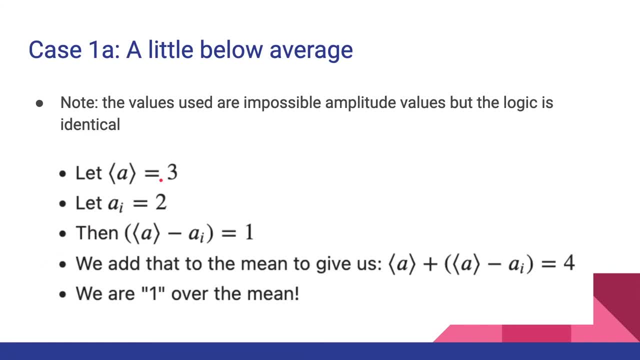 The logic is still the same here. So the average here is 3.. But the amplitude on a particular answer is 2.. So if I do the math here, 3 minus 2 is 1. And then we're going to add that difference to the mean. 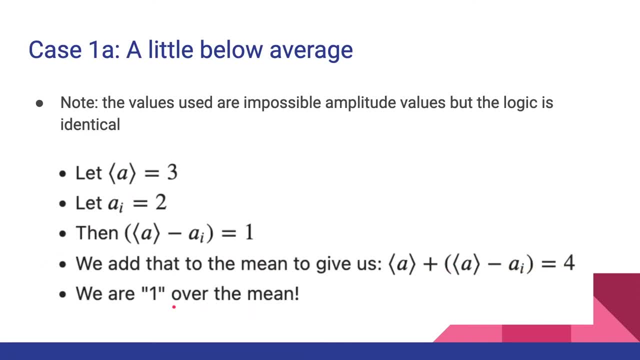 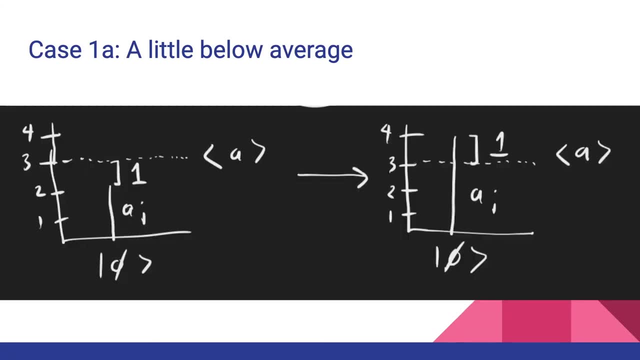 to give us 4.. And, as a result, we're now 1 over the mean. So we were under the mean earlier, And now we've literally flipped over by one unit. So here's a picture You can tell I doodled this myself. 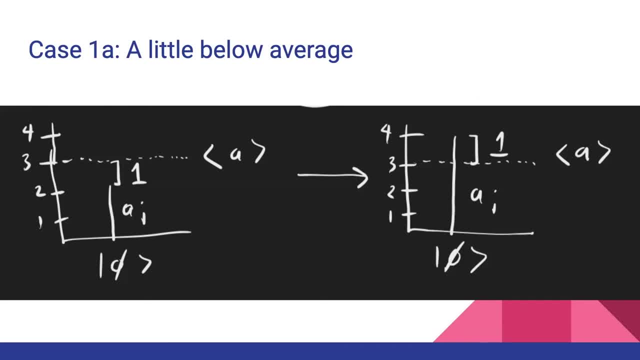 I was a little more proficient with latex, I could have rendered this, And some of the notes out there are gorgeous, But I'm definitely not there yet, So I used to. I used OneNote for this, But this is where we were in the beginning. 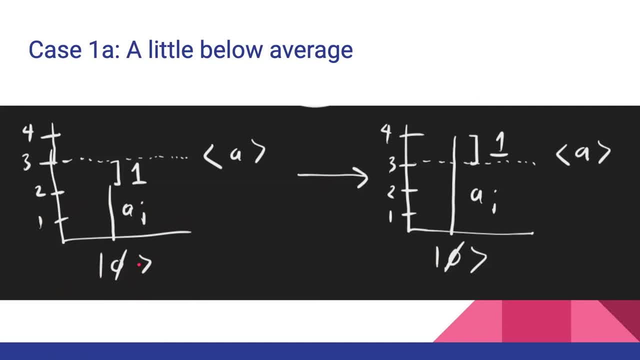 This ket with the very terrible phi in. it is just. I'm just saying this is a random state, So don't worry about the value. But in the beginning we have a sub i which is at 2 here And then the mean is at 3.. 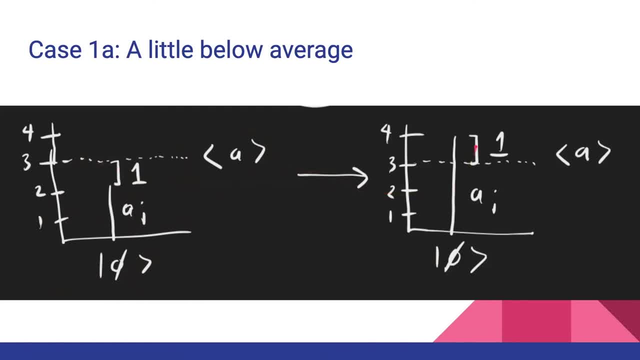 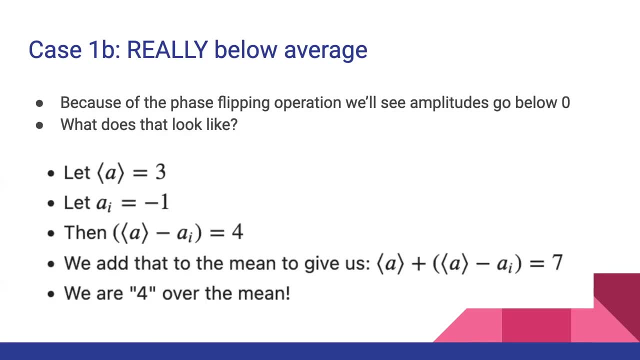 And I apply the operator, I apply the operator And now we're 1 over. So I've just bumped the probability amplitude from being below the mean to being above it. Now, case 1b: It's really below average, like some of my prior class scores. 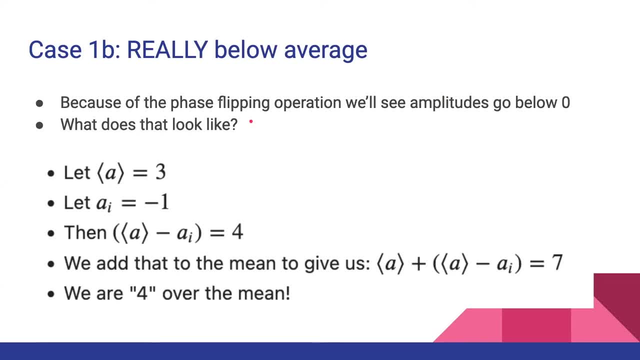 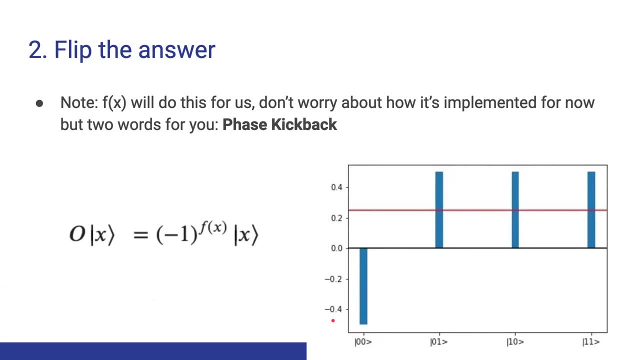 But when we do that phase flipping, you notice that there are amplitudes that go below 0. I'll go back to right here. See now this is negative. So intuitively, if you think, well, if we're a little below the average, 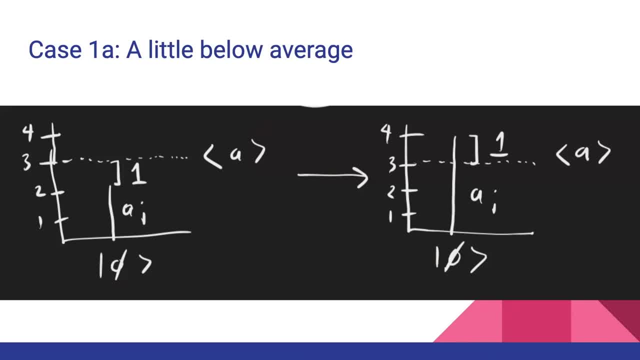 we're going to go a little above the average, And if we're really below the average, then we should go really above the average, And you're right. So we still have the mean of 3.. But I let this equalize. 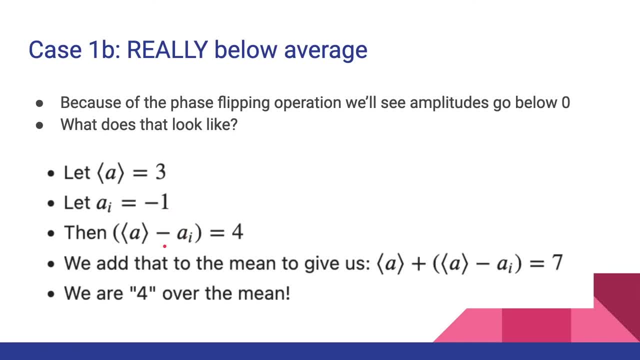 I let this equal negative 1.. So we're below 0. And I do the subtracting here: 3 minus negative 1. That's 4.. And then I add that to the mean, Now it's 7.. So we're 4 over the mean. 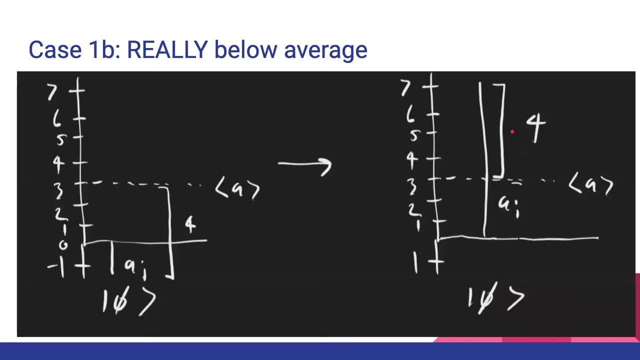 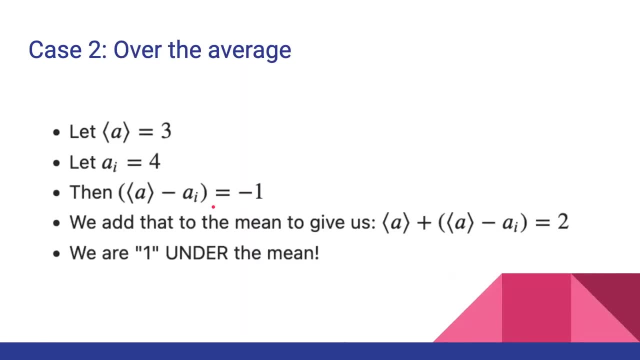 And it's quite a remarkable like this is a huge increase in the probability amplitude. That's what we mean by inversion, about the mean, literally flipping the amplitude over the mean. And then, of course, I have an example here. This is the last case where we're over the average. 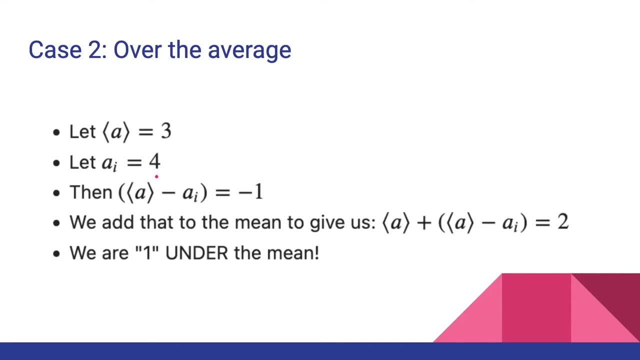 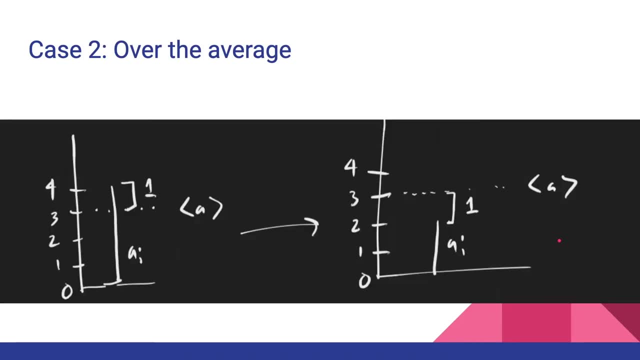 So let's imagine that the average is 3, but a sub i is 4. And we find out, doing this subtraction, that it's minus 1.. So our new probability amplitude is 2.. So now we were over the mean by 1.. 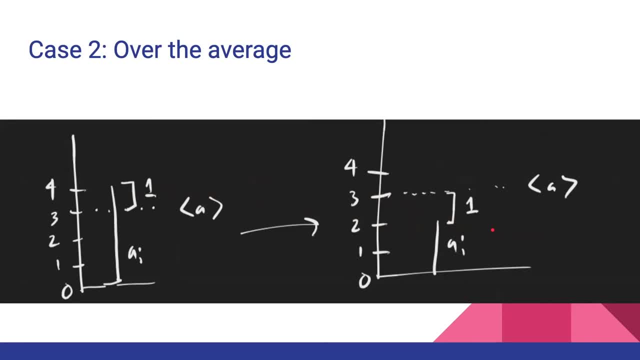 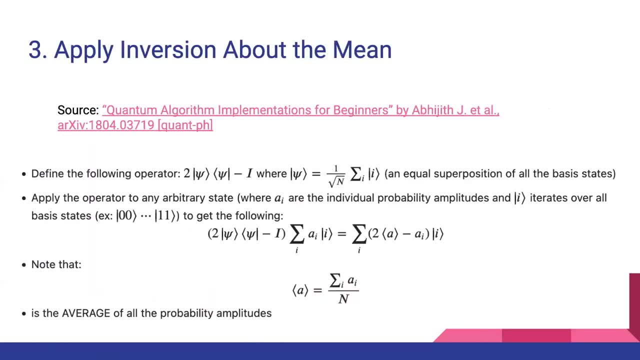 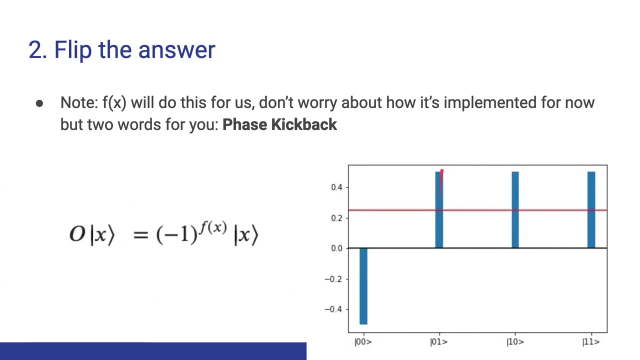 And now we've dropped by 1.. So now we've literally flipped down the mean. So if I take this state here and I apply inversion about the mean, we can just think about this intuitively. Well, these guys, this is over by some amount. 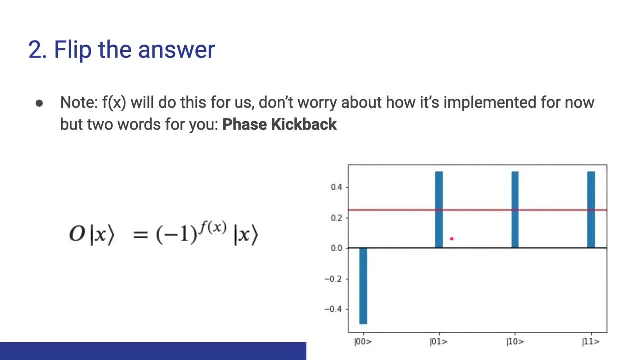 So if we flip it this guy goes to 0. All these go to 0. So intuitively that means that all this amplitude has been kind of pushed to the proper answer here And you can tell this is a huge difference from the mean. 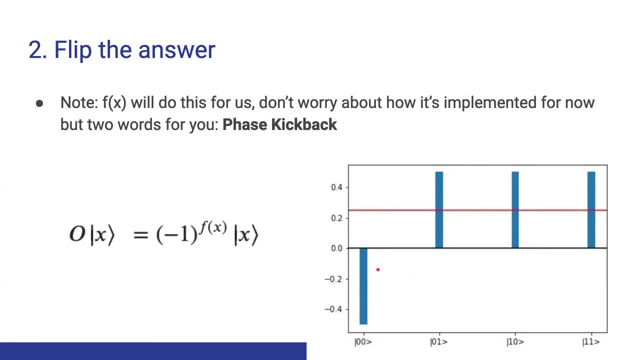 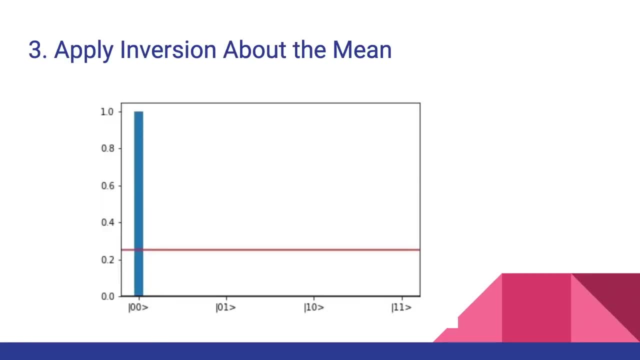 So that must mean that when we flip back up, it's also going to be a huge increase in amplitude. So boom, look at that. Now 0, which I said was the answer earlier- is the only thing you can measure. All the other answers have been annihilated. 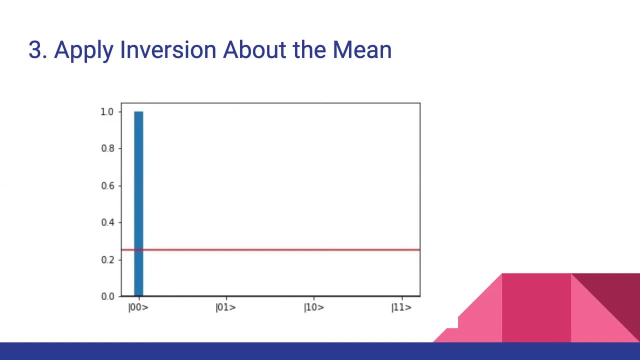 We only have 0 here. This is the 2-qubit example And you notice I only had to apply the operator once. If I have three or more qubits, you'll have to apply the operator more times. In fact, I mentioned earlier it's pi over 4. 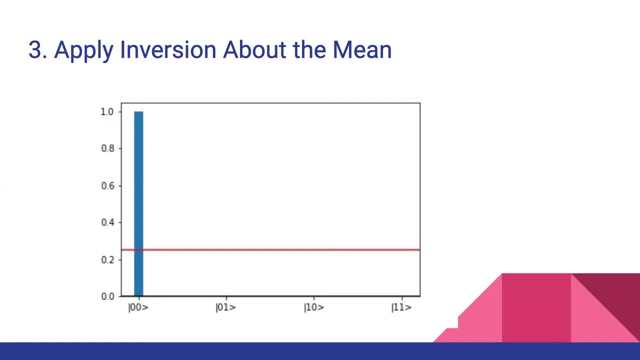 over the square root of n times roughly that amount You have to round down or up because it's pi over 4.. But that'll give you a good ballpark estimate of how many times you need to apply this operation. So for 2 qubits, I think after one operation. 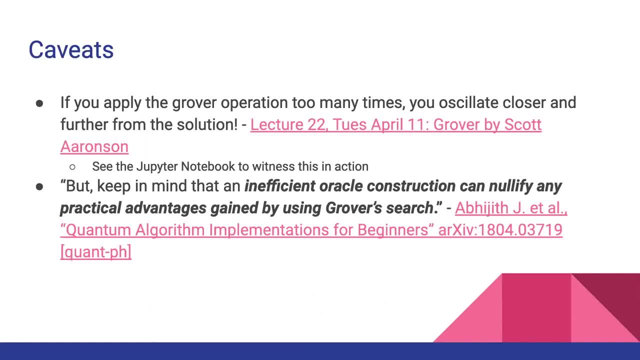 you're pretty much guaranteed the right answer. Ah, now I have the caveats. I'm not trying to sell you guys snake oil. I'm not a quantum hype man. I'm here to tell you as it is. So if you apply the operation I showed you, 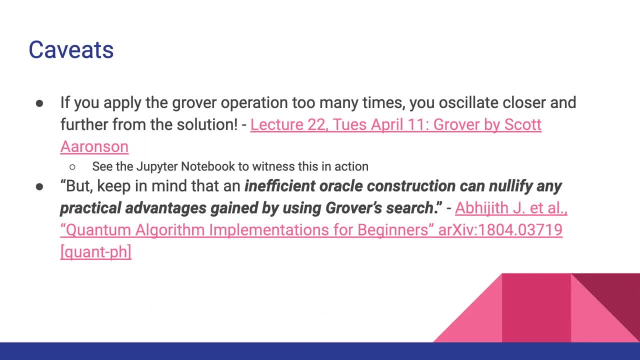 the version about the mean. too many times you actually get further from the right answer. Scott Aronson has a very fun little analogy with cooking. It's not bread, I forgot. It's not fondue, I don't know what it is. 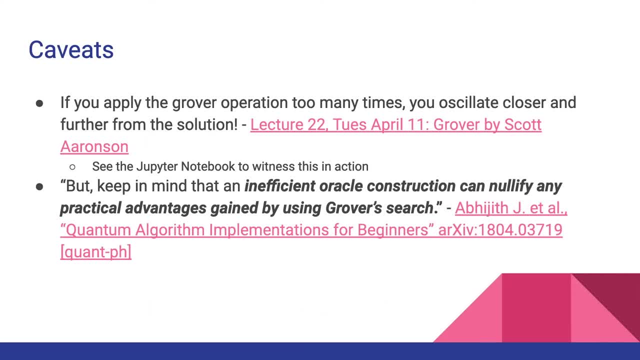 But he said, when you cook bread, the bread rises And you cook it too long and it starts falling back down or something And maybe you burned it. And then but he says like I don't know, It's like in the quantum example. 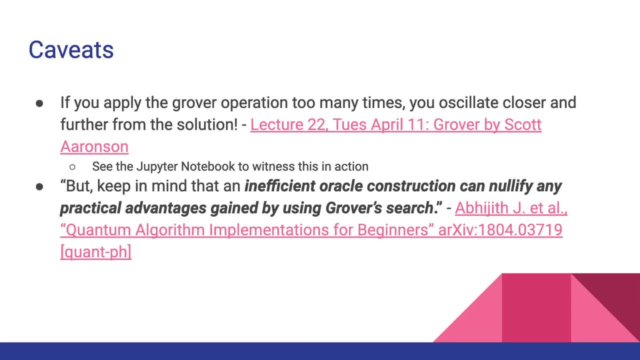 if you keep it longer, it just oscillates to get closer and further, closer and further from the answers You keep applying that inversion about the mean that I was telling you about earlier. Oh, someone in chat has a question Souffle. 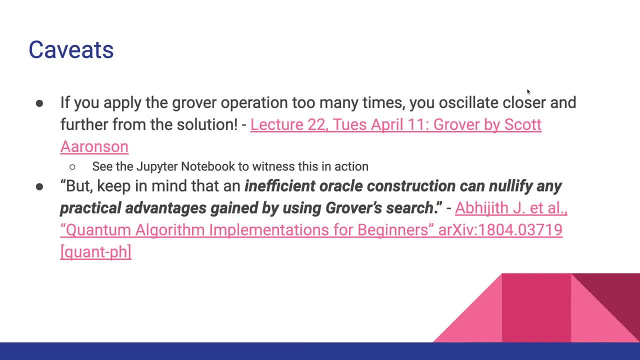 Yes, Kirk McGregor, He's got it right. The example that Scott Aronson gave was souffle. If you put it in, if you're cooking it and you put it in the oven for too long, the souffle will rise and then it will fall. 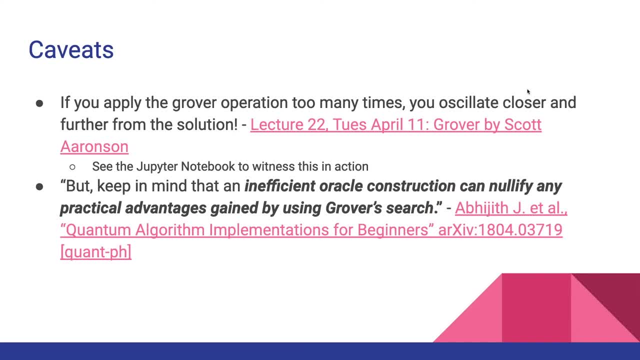 But apparently this souffle repeatedly rises and falls instead of getting burned, Oh whoops. Thanks, Kirk, But there's also another thing I want you to notice. is I kind of said like, oh OK, we can just? 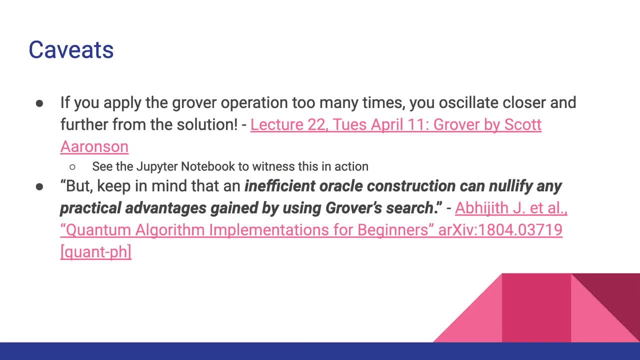 turn f of x into an oracle. And there's a bit of an asterisk you have to put next to that statement, Because to do that requires me to take the problem and translate it into something the quantum computer can understand. And this is from a paper from, I think. 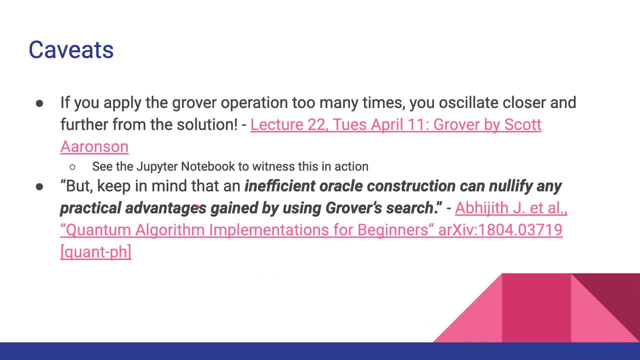 Los Alamos National Laboratory And they said: but keep in mind that an inefficient oracle construction can Nullify any practical advantages gained by using Grover's search. So if my oracle takes a huge amount of gates or ridiculously long amount of time to check the answer, 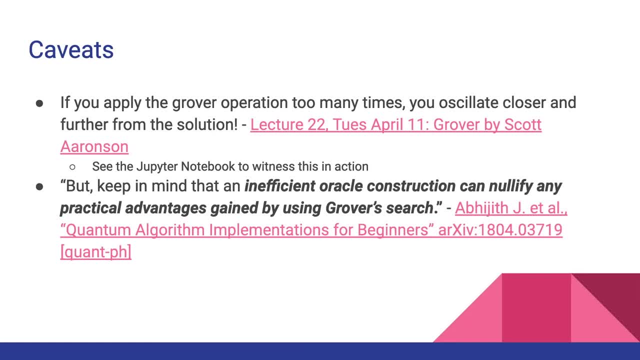 you're not really going to get any benefits on it. So you've got to make sure that when you are implementing an oracle, you want it to be as compact and as fast as possible. So those are the caveats for you. What's going on here? 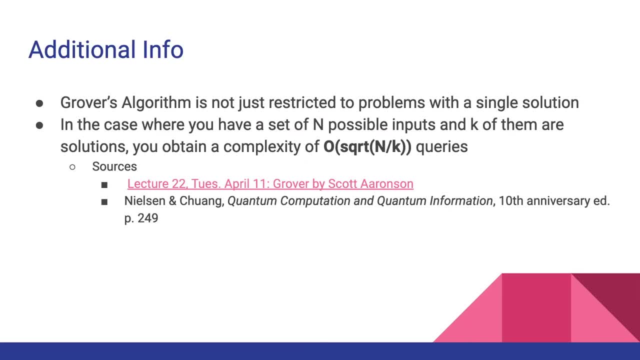 Oh yeah, and some additional info. In that example I gave you, I gave a very friendly example Because it only has one answer. f of x only has one answer. But in the real world you might have a black box or an f of x. 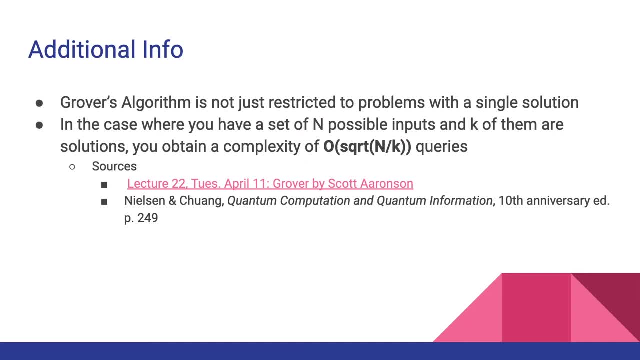 that has multiple answers. So does the Grover's algorithm work for that? And I'm very happy to say the answer is yes. In fact, the complexity, the time complexity for when we have multiple answers is better if you think about it. 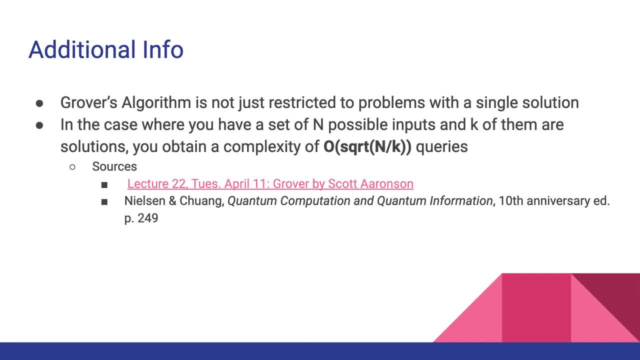 Because now there are two solutions that get the phase And, as a result, we converge faster to two possible solutions. So it's n over root, k clear. So query just means we're invoking the oracle, We apply the oracle. That's what it means to me, say query. 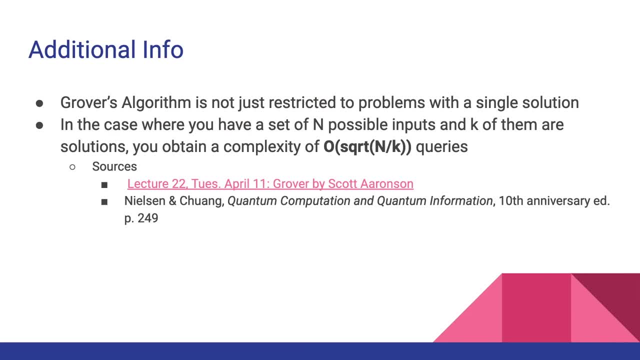 So it's the square root of n over k, And I mentioned how many times you should apply the operator is like pi over 4 times the square root of n over k. Now it's just pi over 4 times the square root of n over k. 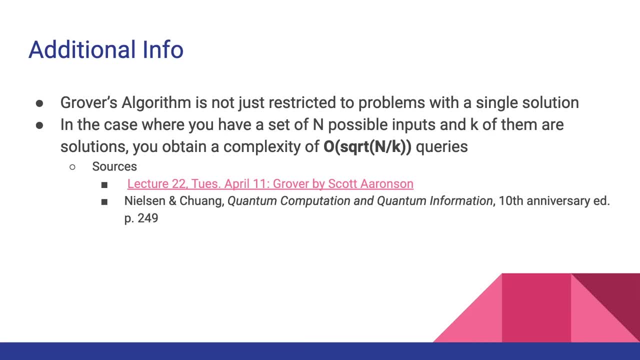 Because the k is the number of possible solutions. Before I go any further now, there's probably a. for those of you that are very observant, you probably have noticed there's a number of possible solutions. I'm not being honest here. 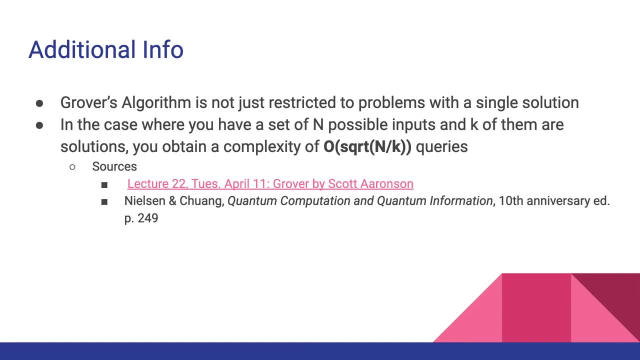 How do you know ahead of time how many answers f of x have In the real world? you may have problems that you don't know ahead of time. excuse me, the number of possible solutions. And it turns out there's actually an algorithmic way. 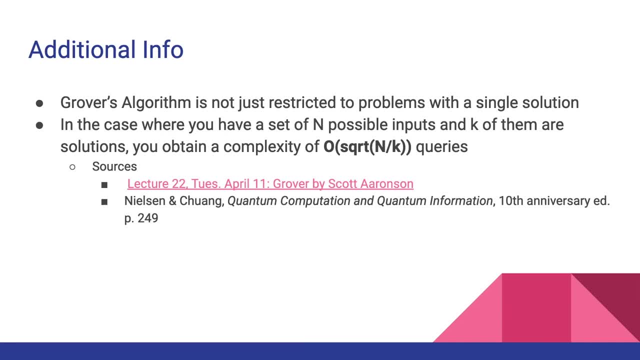 It is very much in some sense like brute forcing, but you're using Grover's algorithm where you pick k to be a powers of 2, I think That was on the Microsoft Azure page- And it turns out that if you do that, 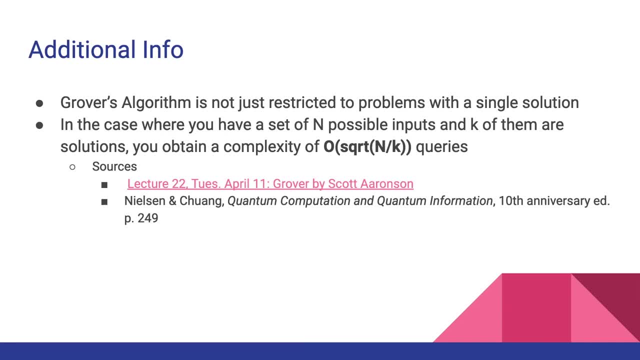 it's definitely overhead but it's still efficient And that's how you can randomly pick a proper k to try and go with. So I think I have it in the notebooks. You'll see that And then implementing the algorithm. OK, cool. 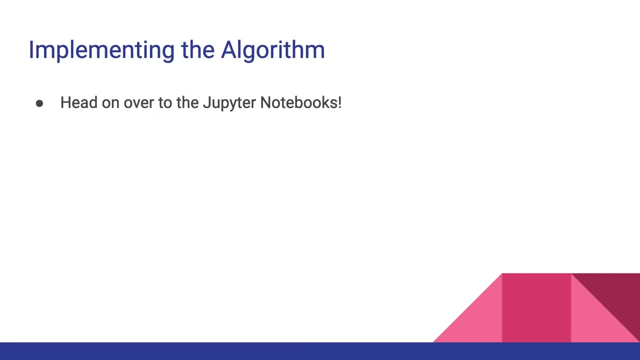 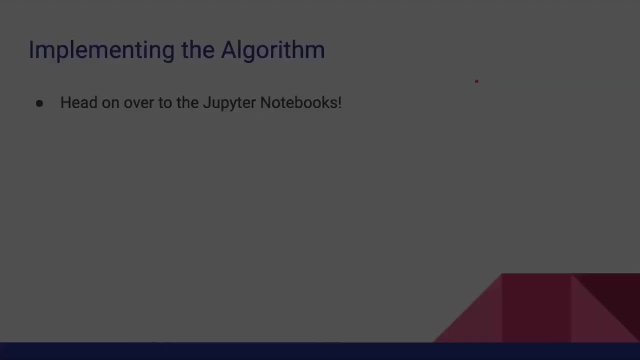 I've blabbered on long enough. I think it's time to let you guys have some fun with some code and some actually rigorous content, I guess. So let me go ahead and end this slide here And I'll give you a brief overview. 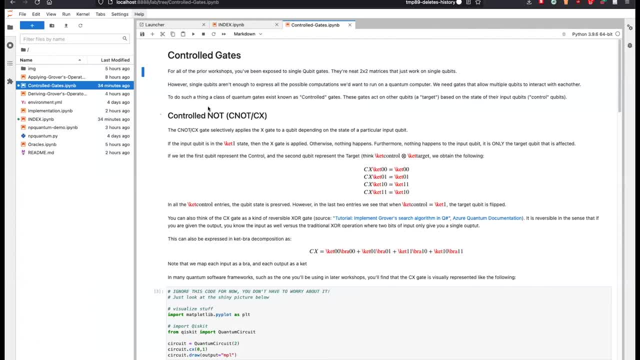 of what these notebooks look like And then I'll show you the URL and let you guys download it and install it. And while I'm here, if you have technical issues, don't hesitate to just bug me. Because I built these. It's my obligation to make sure they work on your systems. 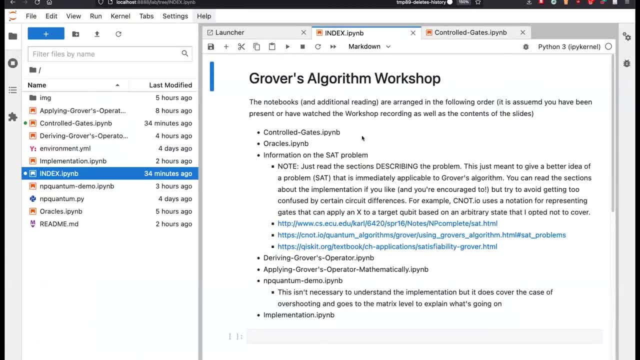 So I do have an index here. It's almost like a table of contents. So I've arranged all these. There's some prerequisite knowledge I didn't cover in the last workshops. Now I've crammed it all into these notebooks And so stuff with controlled gates. 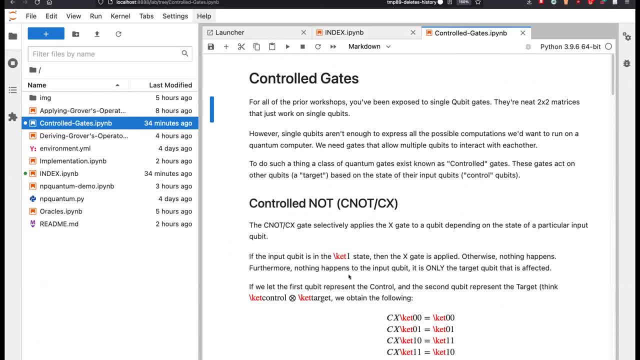 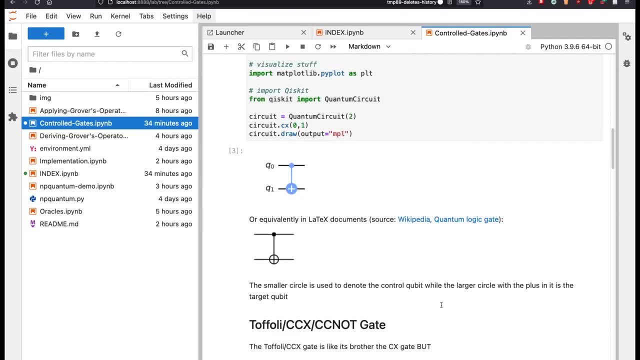 because we'll need these kinds of gates, And you can see there's some rendering. This is supposed to be like an actual arrow, But for some reason my latex is misbehaving. So this is just some preliminary information on some different possible control gates here. 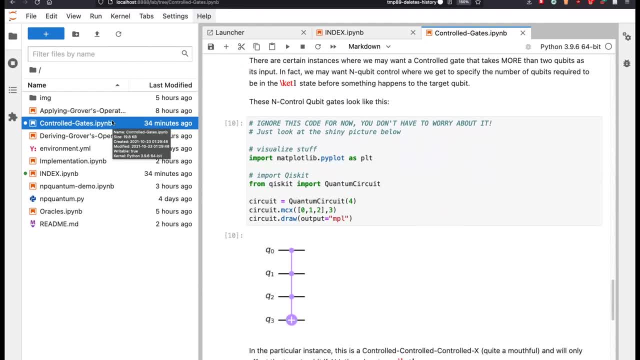 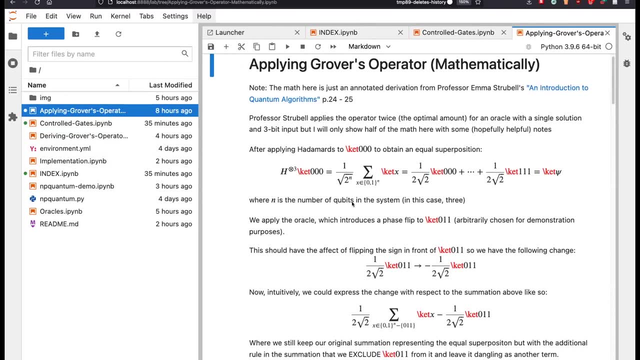 And you'll notice my treatment in terms of the math was intentionally light Because I've put all the labor of showing the math in here. So how to mathematically apply the operator as well as how to derive it, So the derivation for it. 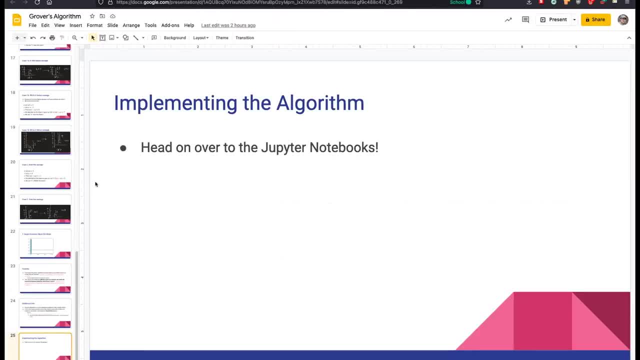 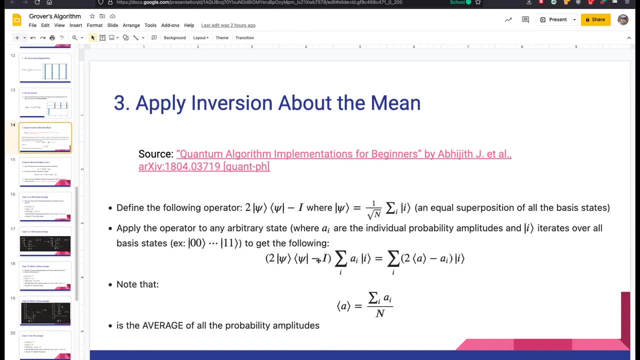 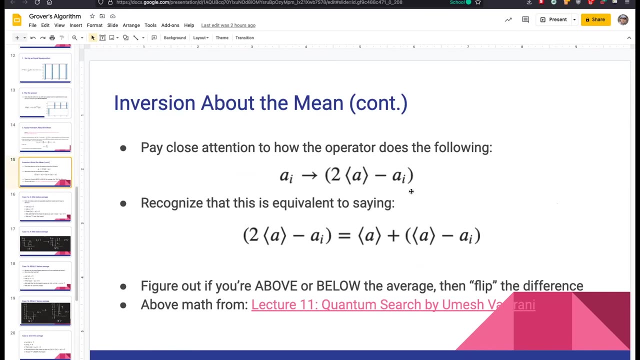 So, because you might be thinking how the heck does, let me see if I can pull it up here. Yeah, How the heck do we go from this to getting this behavior, going from a sub i to 2 times the mean minus a sub i? 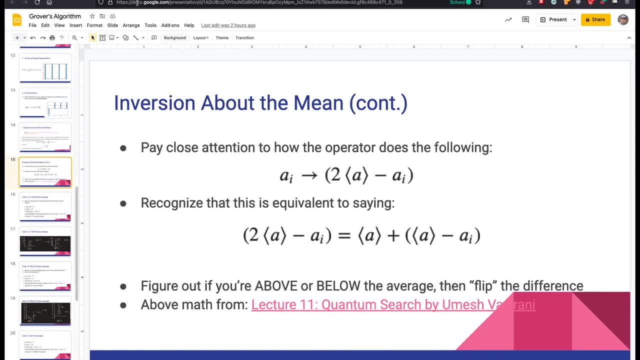 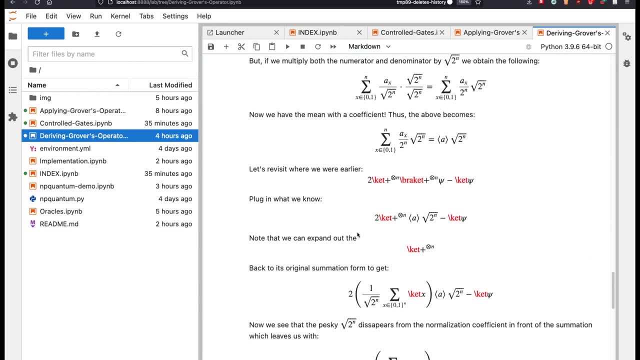 I intentionally omitted that from me just blabbering on, But I've written what I think is a helpful explanation in this notebook. So there's plenty of math here And I- This is. I want you to think of this more as like a. 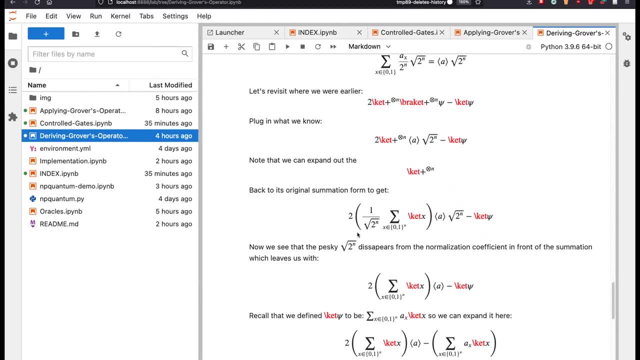 Because this is another professor's work out there I just annotated. I've added some comments that I think would be helpful for you guys to figure out, Because a lot of times these courses are oriented towards grad students And they omit many a number of steps. for the sake of brevity, 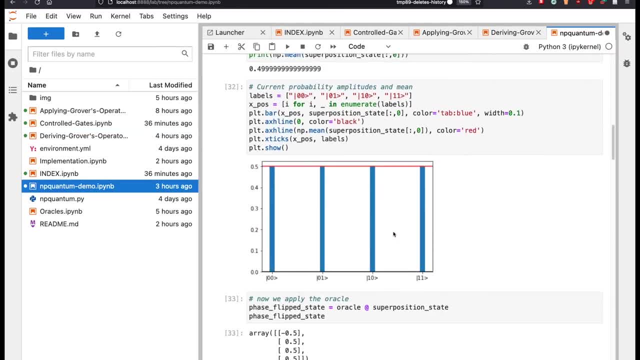 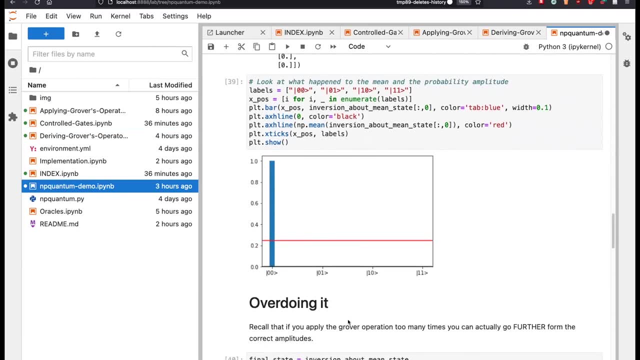 And then from there I also have. So remember those nice diagrams. Well, here they are, So you can go ahead and figure out how I generated those diagrams and see the, see the process for yourself, And I have a section here. This is the fun little thing, overdoing it. 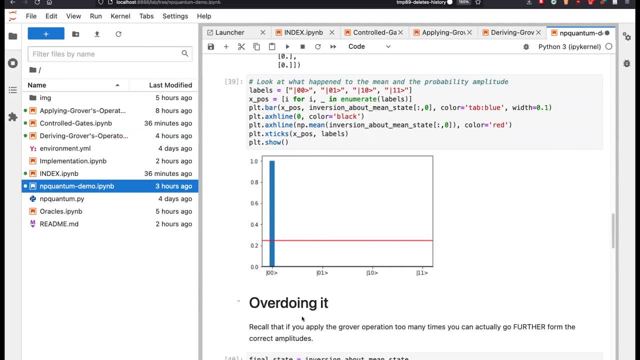 So remember, I told you it's very important that you don't apply the Grover operation too many times. What exactly does it look like when you apply it too many times? Well, let's say we start from here. We're already at our answer. 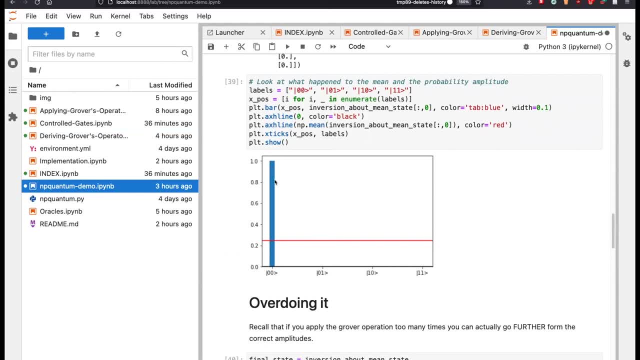 Why bother applying it again? Let's say, maybe I look for a coffee break And I let the intern write the code And he decided maybe if I put some more operation it'll be better. And it turns out we apply the oracle again. 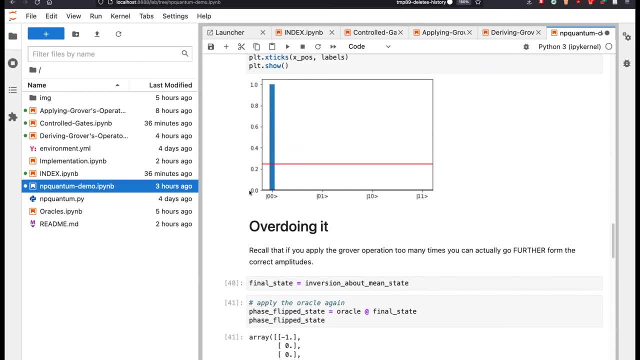 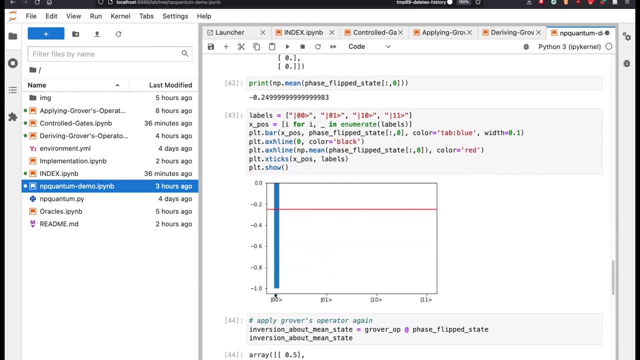 So now we're upside down. You see, here we were from 0 to 1. And now I flip it. So now we're from 0 to negative 1.. No problem there. If I were to measure it now, we'll still. 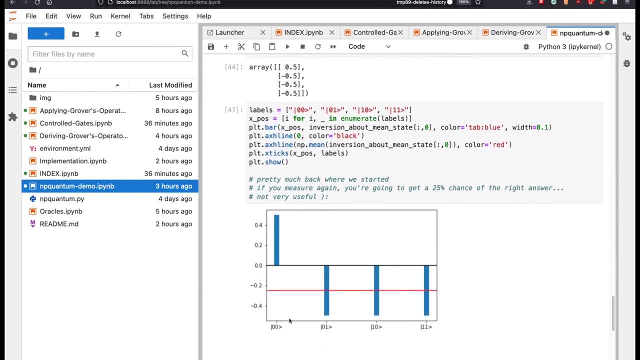 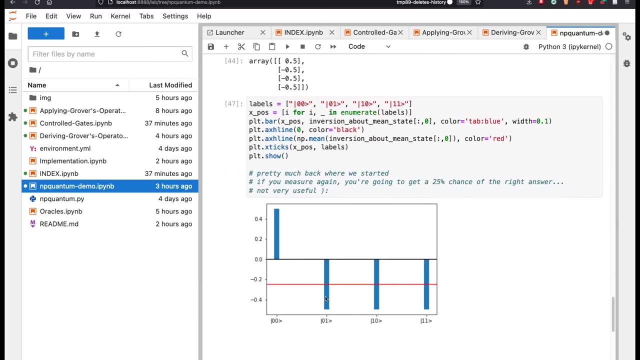 get 0 as the final answer. But I apply the inversion about the mean And I've just undone all the work that I did earlier. So now we're back in the equal superposition state. The phases are a little flipped here, But if I measure it it's still an equal chance. 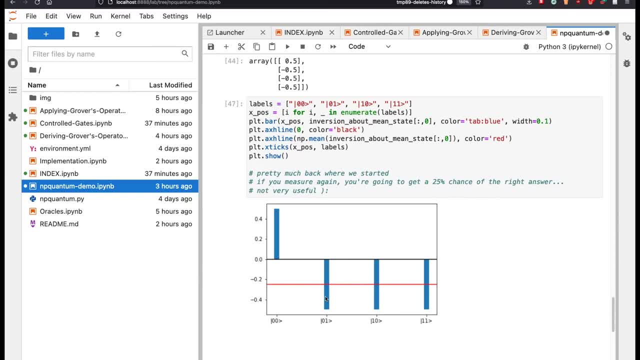 I'm measuring every other answer, which means I've literally undone all the work I did earlier. So that's the consequence of applying the Grover operation too many times. is you literally undo your work? Of course, if I applied it again? 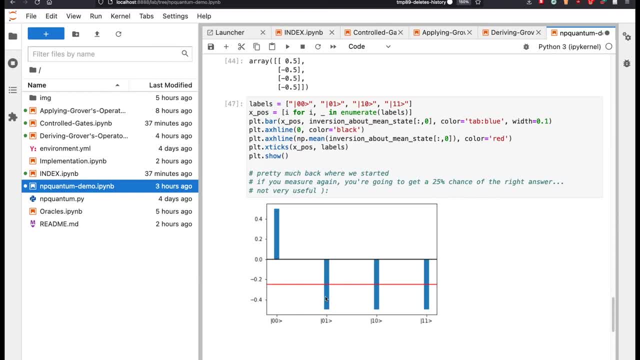 I could go back to my answer. But if you apply it again, you better have a very stable quantum computer, Because the problem with quantum computing right now is: errors creep in. So the first iteration: there's a little bit of error, And then I apply it again, and again, and again. And the error starts to build up to a point. And then I apply it again and again, and again, And the error starts to build up to a point. And then I apply it again and again, and again, And the error starts to build up to a point. 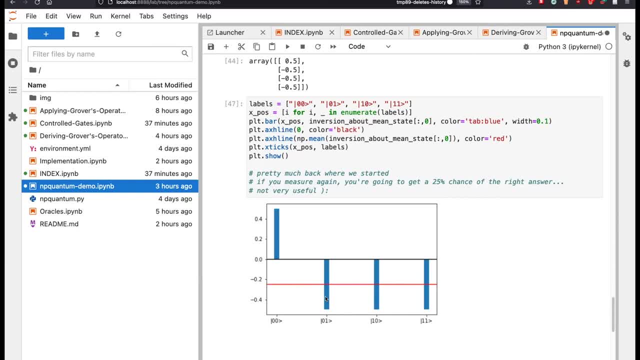 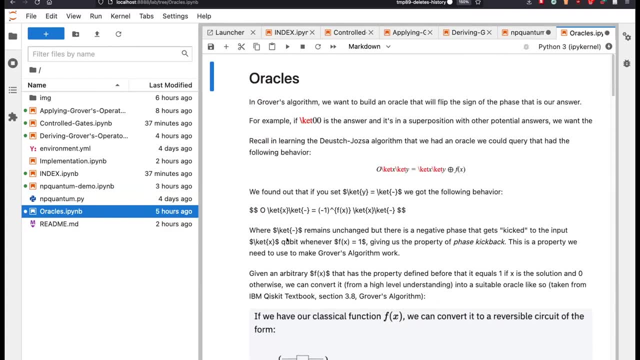 And then I apply it again and again And the error starts to build up to a point Where eventually, your answer is just totally wrong. just because the error creeps in. It builds up over time, And I also have. let's see, I have a section here on oracles. 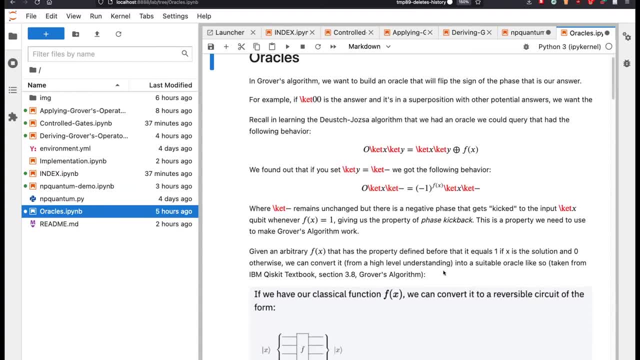 So I told you like: oh yeah, f of x, We could do some operation with f of x. Well, I have here the details, Like OK, here's how you should think of them And here's how, oh, and I introduce you guys. 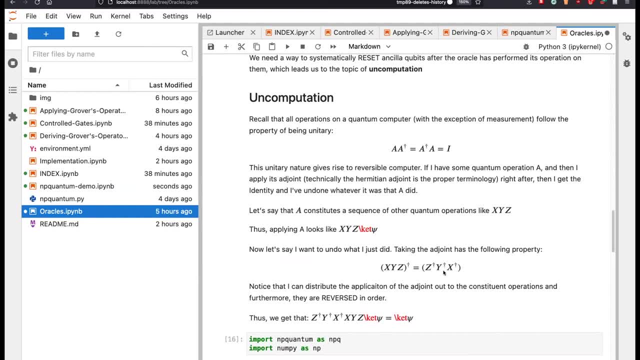 to uncomputation. So occasionally the oracles will need some additional working space, like an additional qubit or two, And those additional qubits don't contribute to the final on f of x. Well, they do contribute to the final f of x. 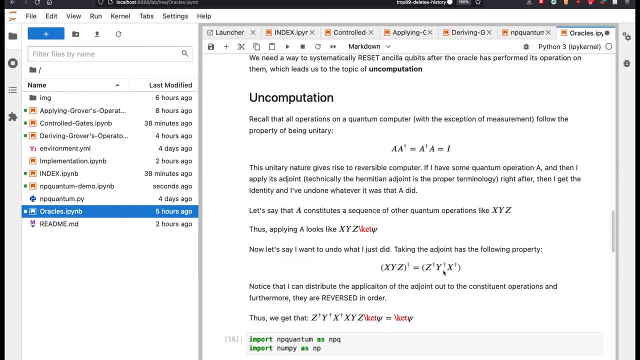 But they're just kind of sitting there. It's almost like when you're taking an exam and you need scratch paper. Think of it like scratch paper for the quantum computer. The problem is that scratch paper gets reused again and again and again. 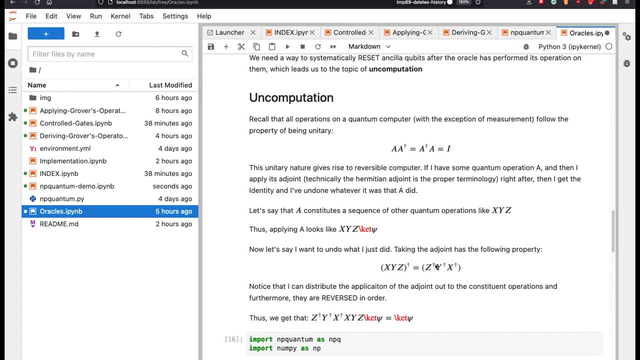 And if there's old stuff on the scratch paper, the quantum computer is going to mess up your future results. So we have a procedure known as uncomputation. We can literally undo What we did earlier and reset the state of our qubit. 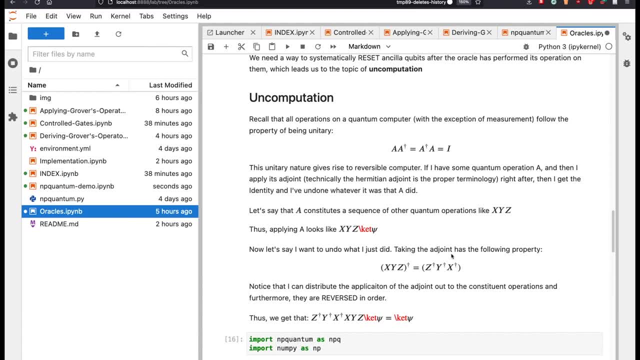 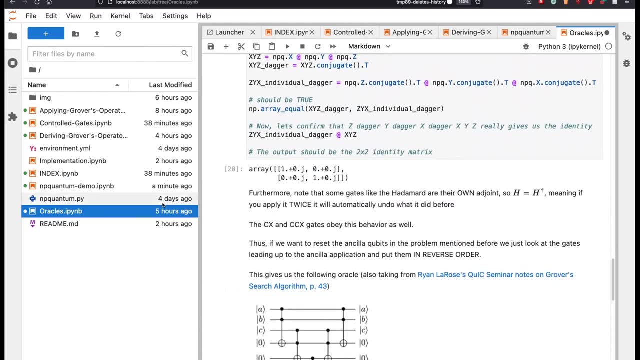 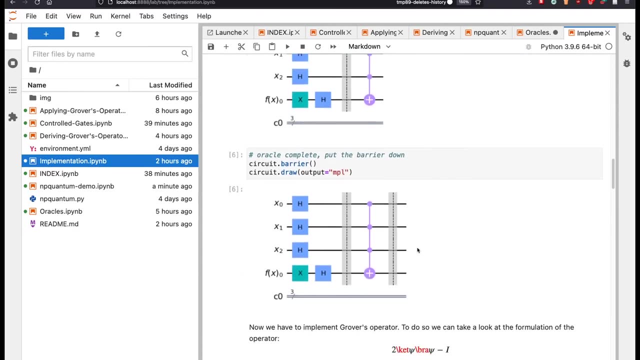 And mathematically it's a very simple idea, very elegant, And I hope my explanation is as equally elegant as well. And of course, the sort of cherry on top here is I do have an implementation, So you will see what an actual oracle looks. 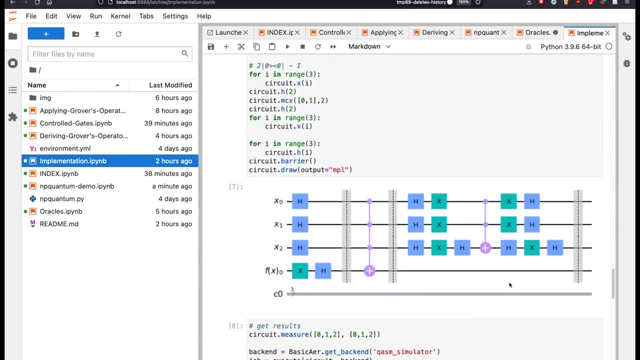 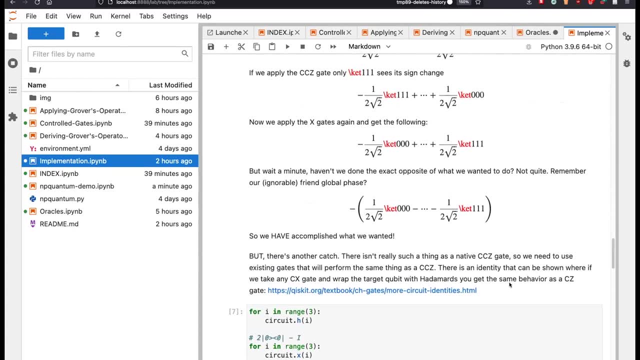 like on a computer, and how this whole thing works, And I'm going to show you how to do that. And once again, I'm just giving you an overview of the notebooks. The actual meat and potatoes are all in the latex which, for some reason, 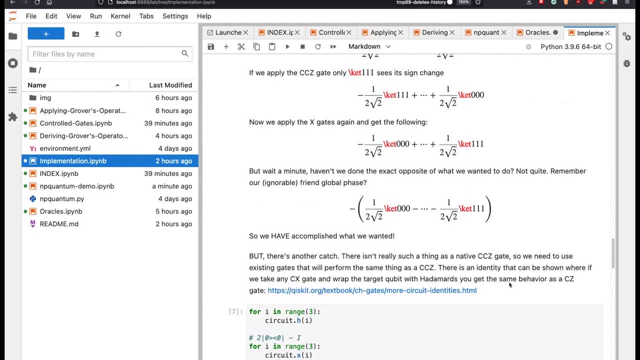 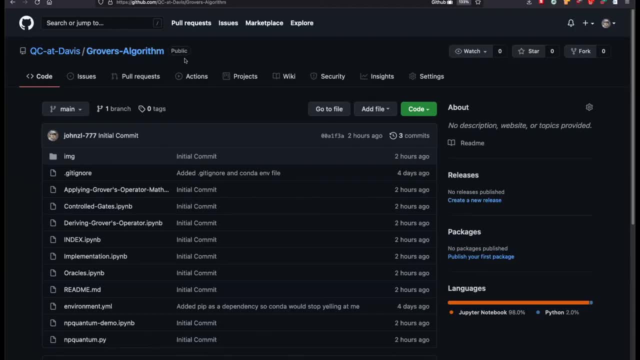 does not want to render properly on my computer. So, with that being said, that's sort of the end of what I have to present to you. I encourage you to let me give the URL here. I don't know if you can. That's kind of tiny here. 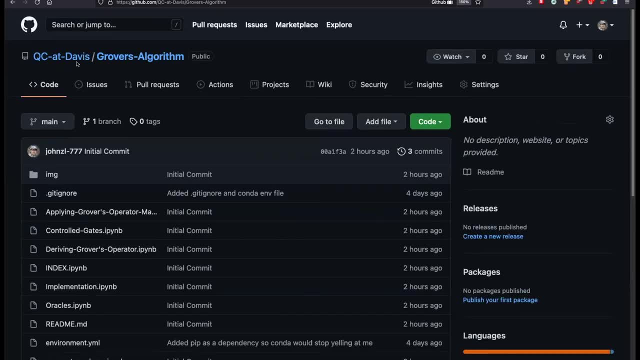 Maybe, if I can zoom in, that'll make. Or you can go on GitHub here and look for QC at Davis And you should see Grover's algorithm as one of the repositories. But in the meantime, if anyone has questions, feel free to ask. 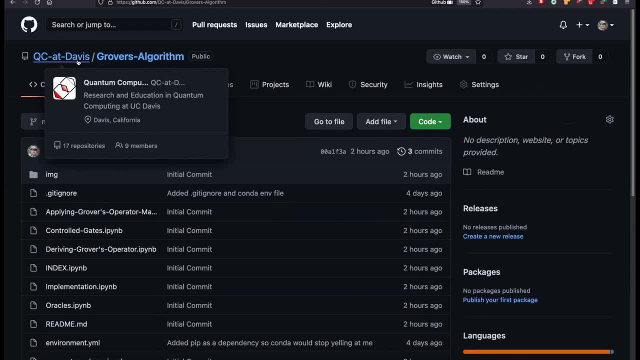 If the latex still doesn't render properly on your systems as well, let me know I can push a fix for it.